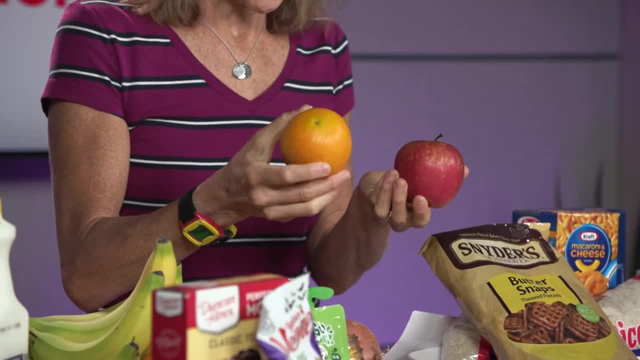 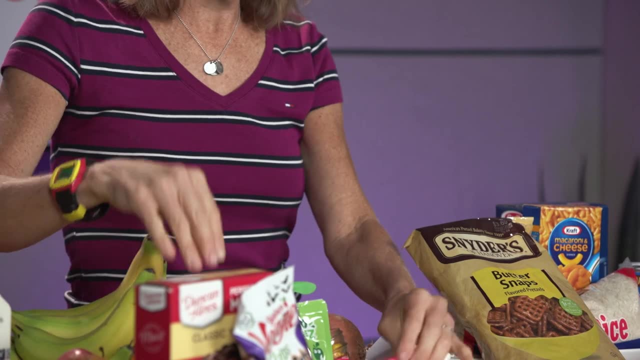 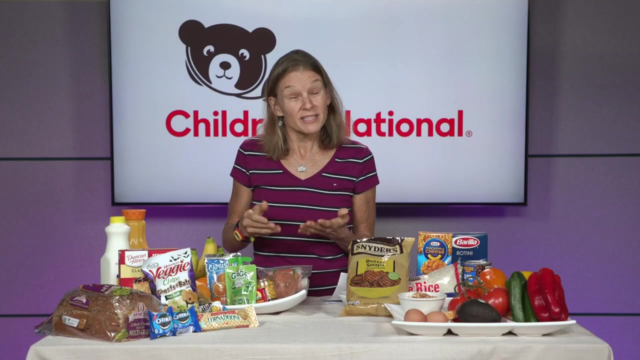 Apples, oranges, all the fruits have carbs, even fruit juices like this Capri Sun. Then we also have dried fruit. So, whether it be raisins or dried mango, more carbs in these foods. Most veggies do not have carbs, However, there are some starchy veggies that do This. 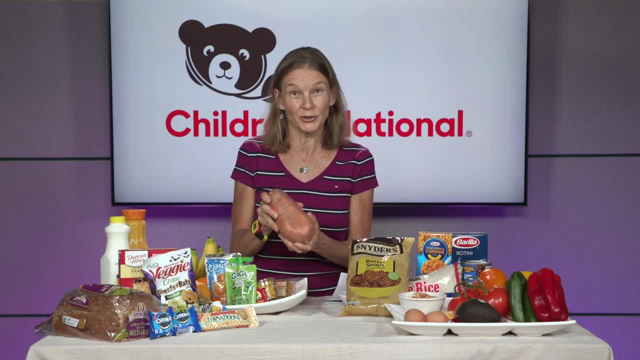 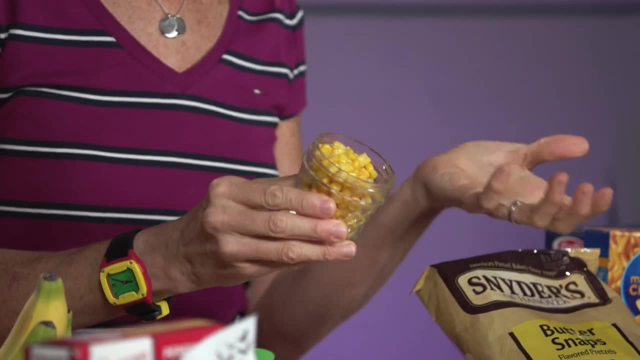 sweet potato, for example, is one that has a good bit of carbs, So you'll need to count that in your calculations as well. That's going to raise your blood sugar level. So a little bit more than a half, a little bit less than a half Corn, whether it be on. 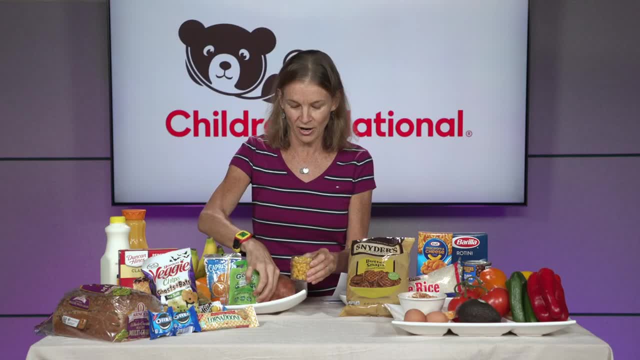 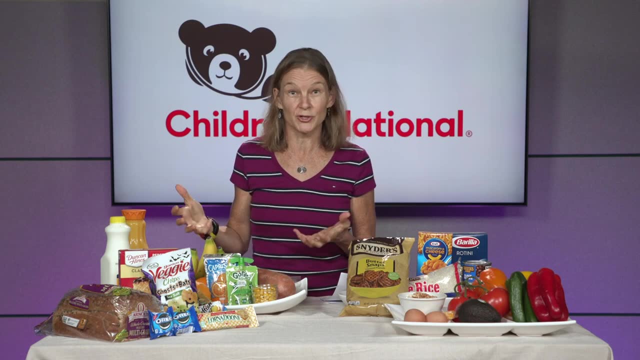 the cob in the can. frozen corn will always have some carbs. Also, regular potatoes and green peas have carbs as well. So while these fruits and veggies are super, super healthy and you need to keep them in your diet, it's important to know how many carbs are in them. 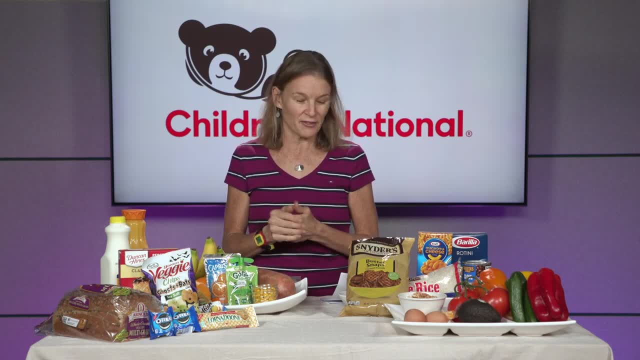 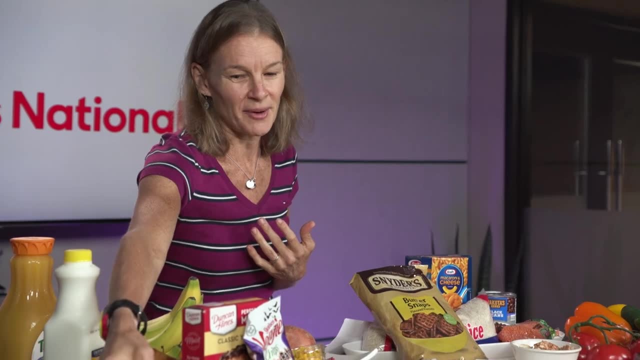 when it comes to calculating your insulin. Other foods that have carbs: anything with flour or sugar is going to have carbs, So that starts with. we got some bread over here, So bread has some carbs. There's flour in bread Even. 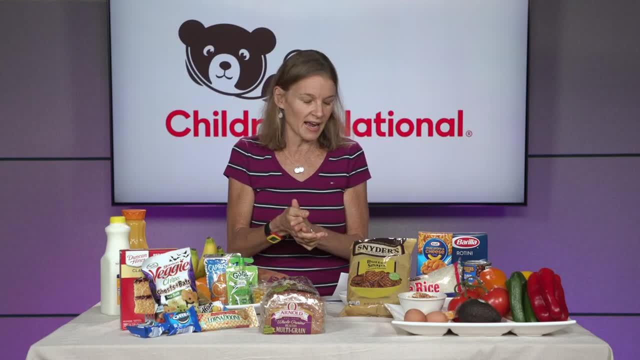 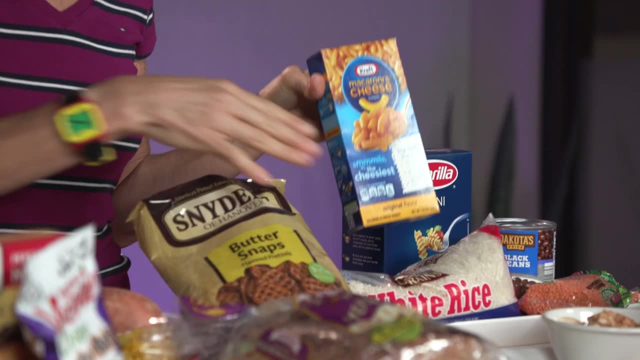 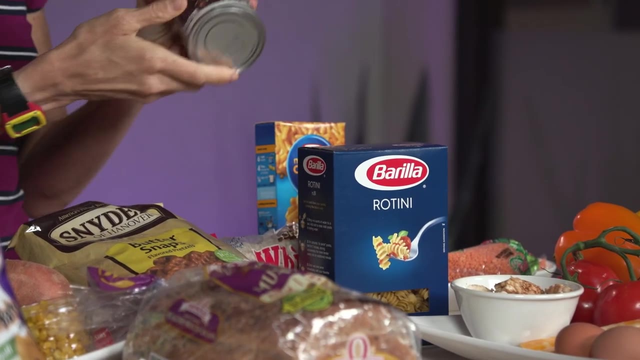 if it's gluten-free bread, it still has rice flour, so that's going to have some carbs. Snack foods have have carbs. They have flour in them. Mac and cheese, rice pasta- All of these foods have carbohydrates. Also some beans and 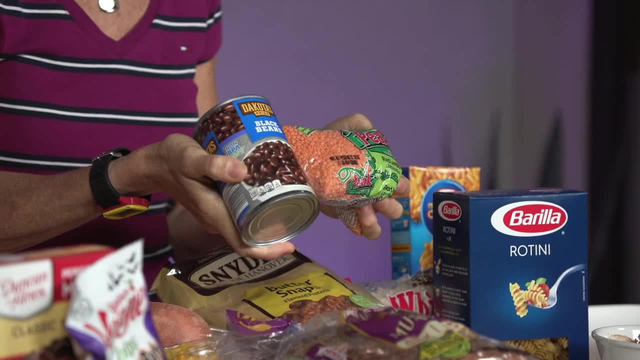 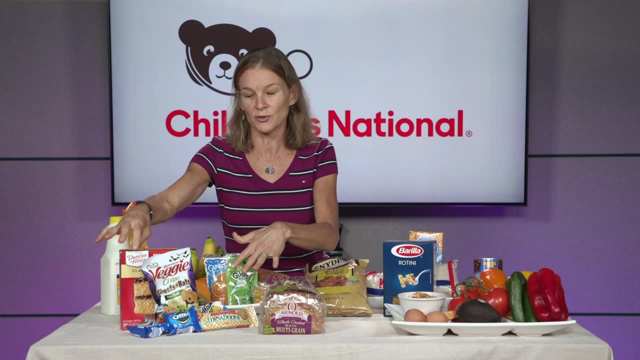 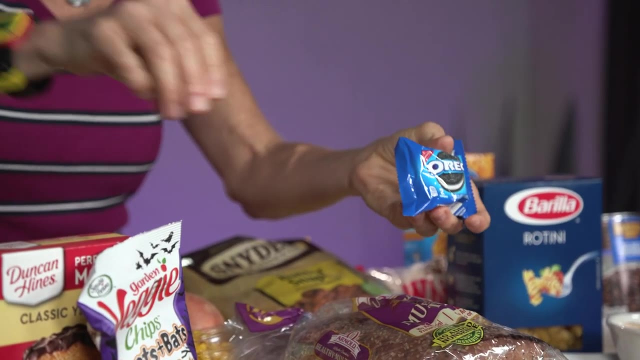 lentils have carbs as well, So these are other foods that you're going to need to count in your carb calculations. And then the really good stuff, the snack foods and the dessert foods. So cookies, goldfish crackers, more cookies, cakes. 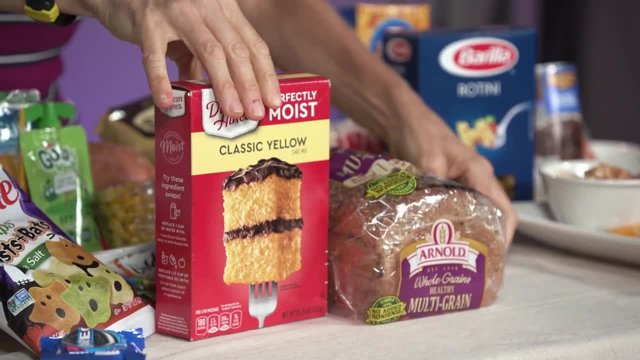 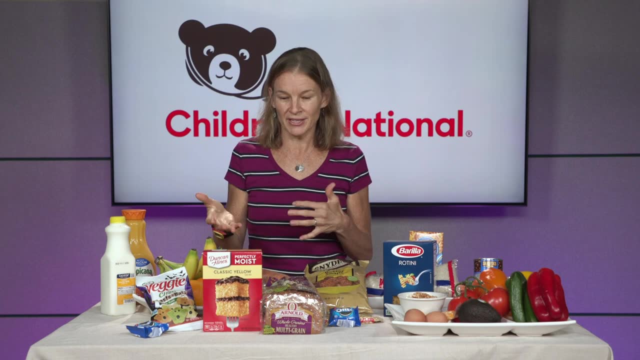 These foods all have carbohydrates as well. So, when it comes to calculating your insulin doses, you're going to want to know which of these foods are in your meal, and then we're going to talk about how to figure out how much insulin to calculate for those foods based on that. 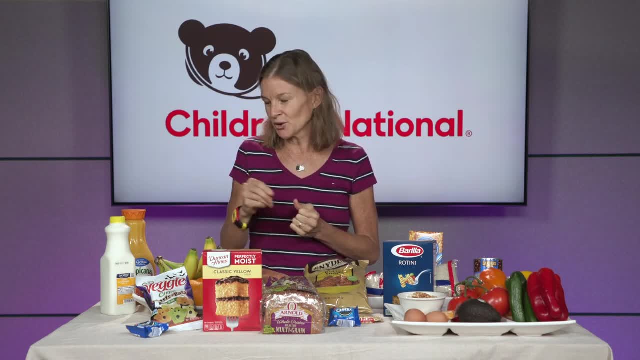 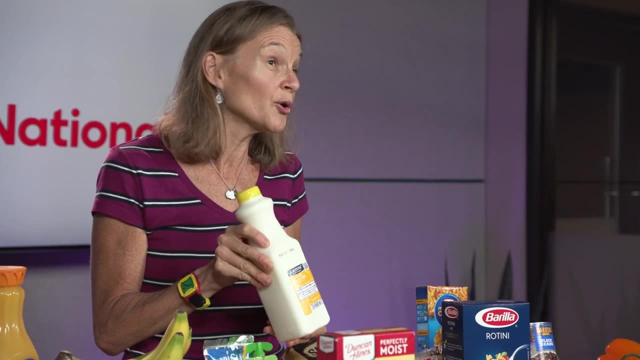 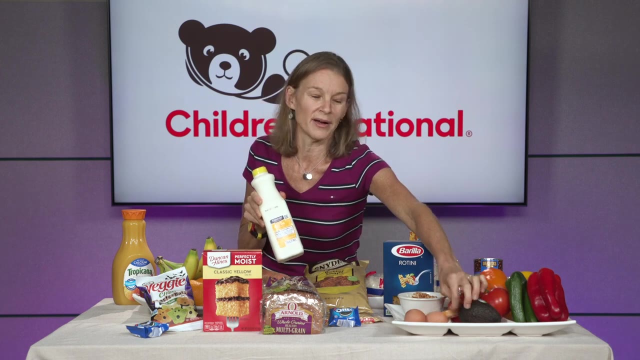 So you're going to want to know how much insulin to calculate for those foods based on the carb content. One last little category that does have some carbohydrates, some dairy foods. So this milk will have some carbohydrates. Also, yogurt has some carbohydrates, But then, to keep it interesting, there are 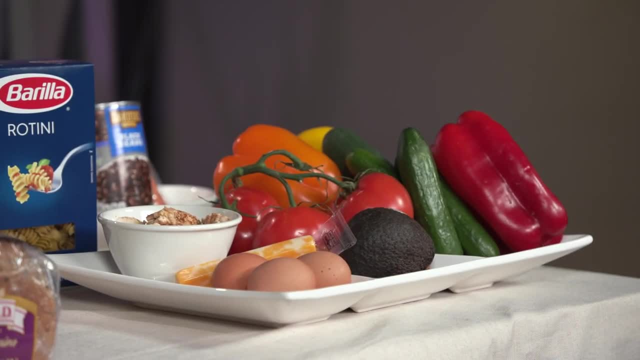 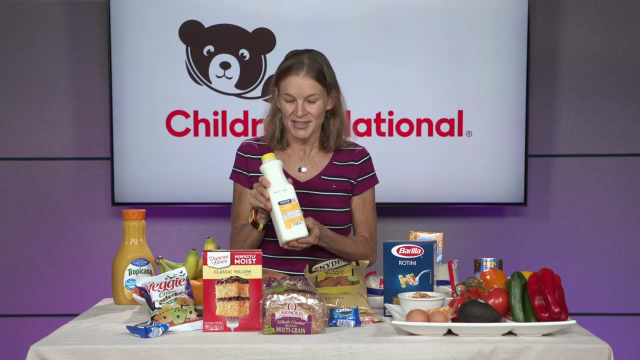 some dairy foods that don't have carbohydrates- Cheese is one. So if you can have a cheese stick which has no carbohydrates, but when you have a glass of milk that does have carbohydrates, So it gets a little tricky, but you can keep that in mind. So the next thing we're going to do is we're going to do some 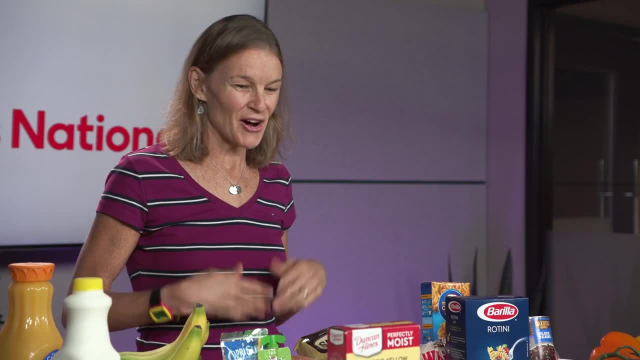 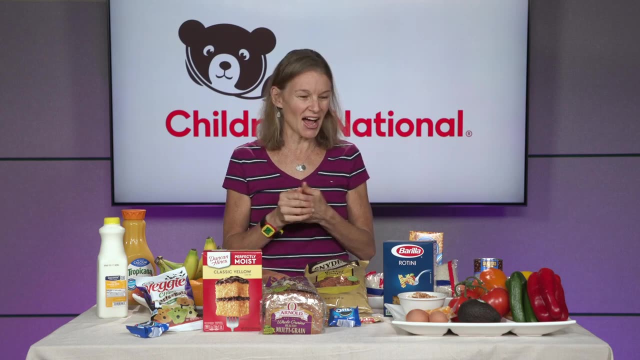 sample meals and calculating carbs, and you're going to see it's a lot easier than you think, All right. so now that you know what foods do have carbohydrates, you might be wondering: are there any foods that don't have carbohydrates? and the answer is yes, All these veggies that don't have the starchiness to them. they 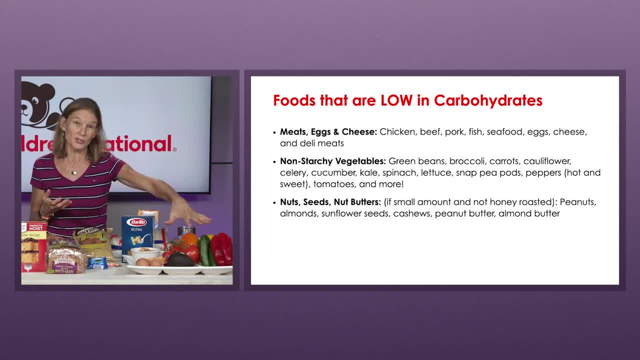 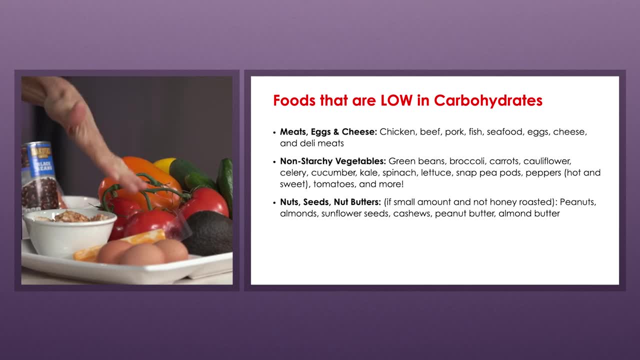 are basically carbohydrate free. They're very low in carbohydrates, So these foods don't have carbohydrates and they won't be counted in your carb count when you're trying to figure out insulin Food. so eggs, cheese, meats- they don't have carbohydrates either, So they won't. 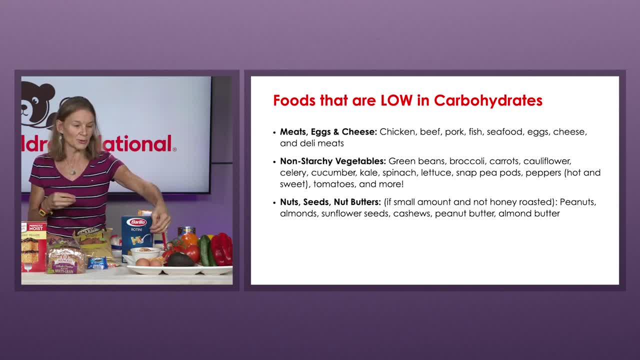 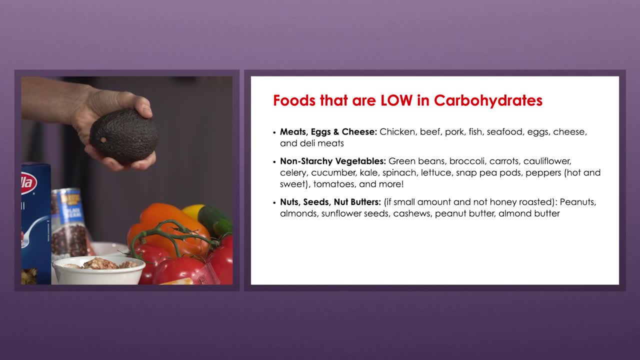 count into your carb count and you're going to see that when we do our sample meals. Avocado is another another. it's actually a fruit, but it's another food that doesn't have carbohydrate. I guess it's the only fruit that doesn't have. 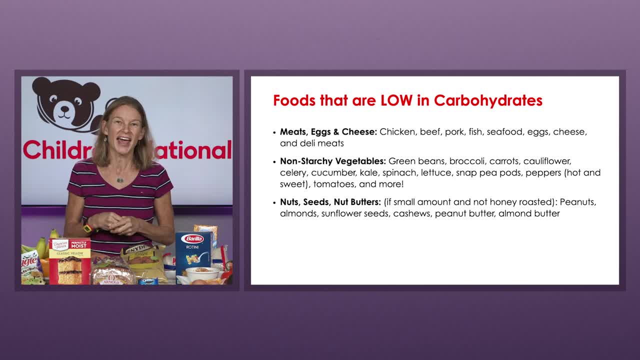 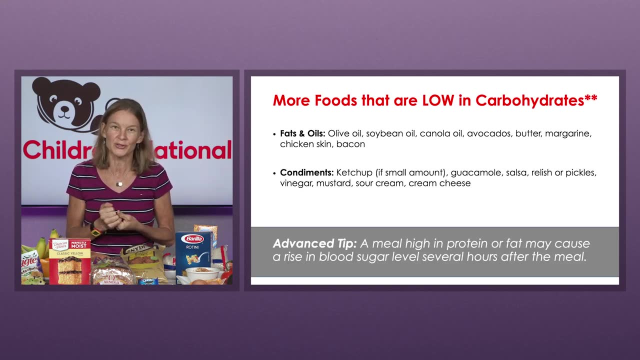 carbohydrates significant enough to count in your carb counts. Other foods include nuts and seeds and nut butters like peanut butter, almond butter. They have some carbohydrates, but low enough that they don't typically raise blood sugar level very much and you typically don't need to count those foods in your carb counts. And also condiments, So mayonnaise. 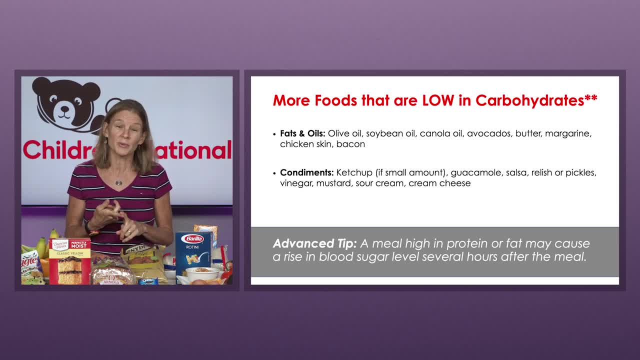 hummus, mustard. even ketchup- Even though it's sweet, we typically don't eat enough ketchup that it's going to be a significant source of carbohydrates when we're doing our calculations. All right, so these are all the foods that might. 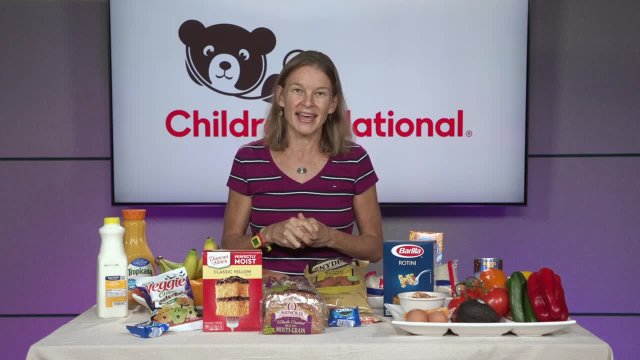 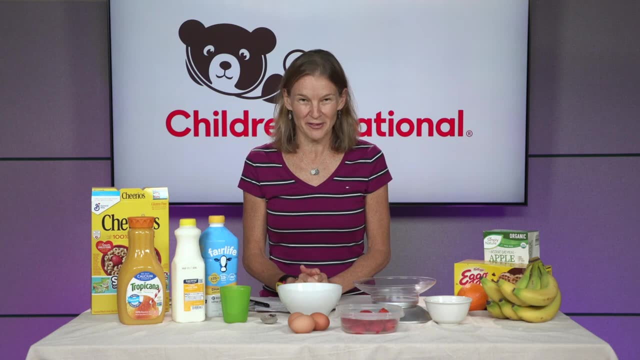 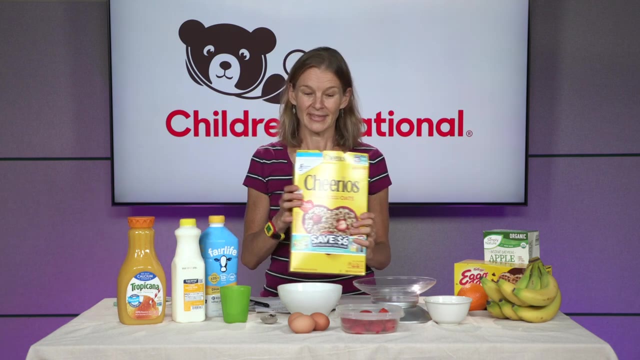 make up your your day. So next, what we're going to do is do some sample meals so you can see how simple this really can be. All right, now that we've figured out which foods have carbs, let's eat breakfast. For breakfast today, I'm going to have some Cheerios cereal. I'm going 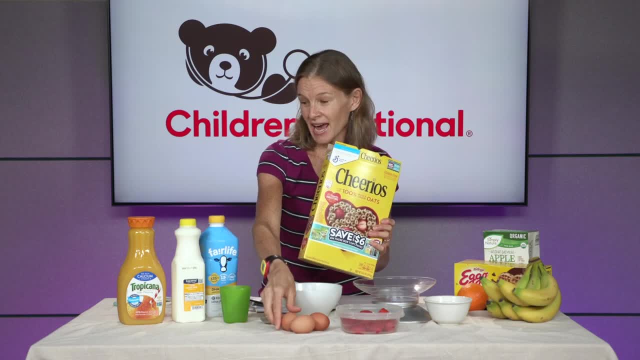 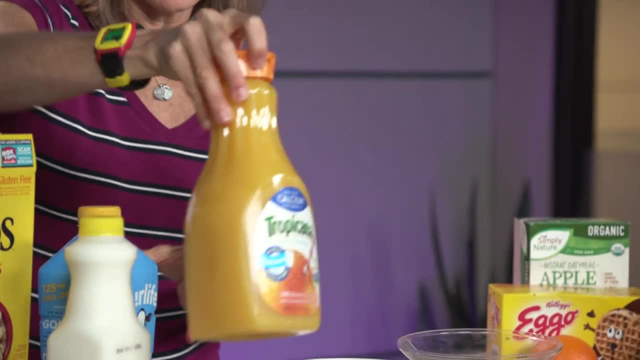 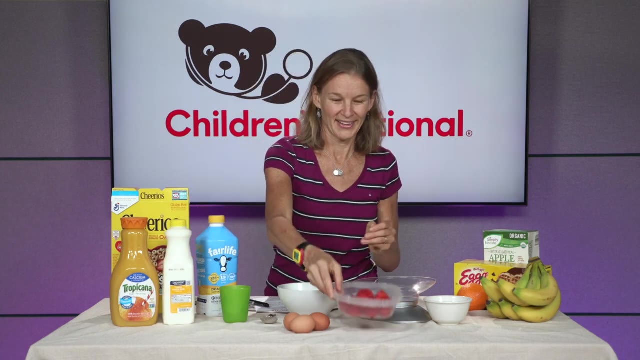 to have a hard-boiled egg, I'm going to have some orange juice, I'm going to put some regular milk on top of that cereal, And then I'm also in the mood for my favorite fruit, which is strawberries. All right, so now there are three ways that we can figure out carbs in these different 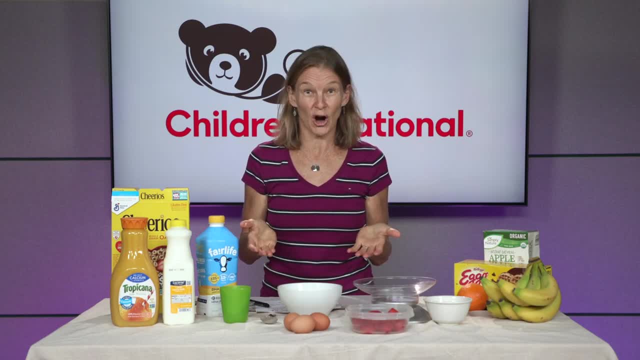 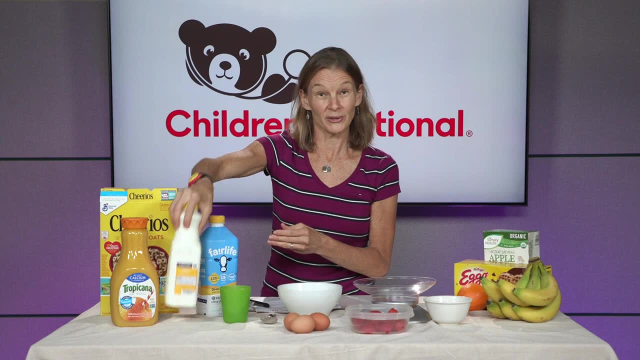 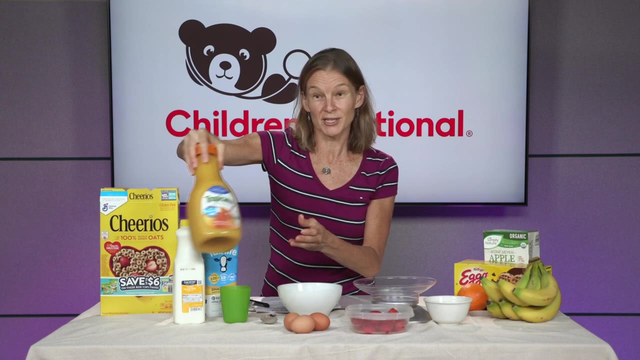 foods. First of all, let's talk about which foods have carbs. Cereal: it's got grains in it, so that has carbs. The milk: that's one of those dairy foods that has carbs, so I'm going to need to count those carbs as well. The orange juice is. 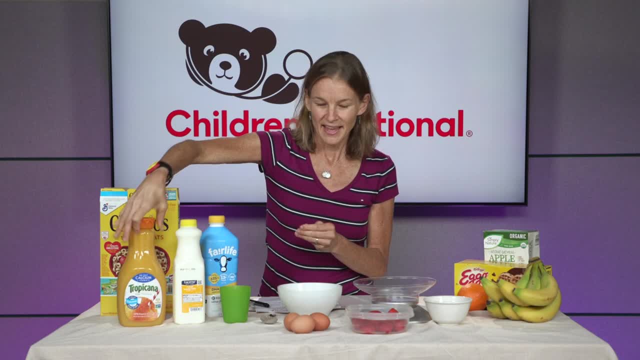 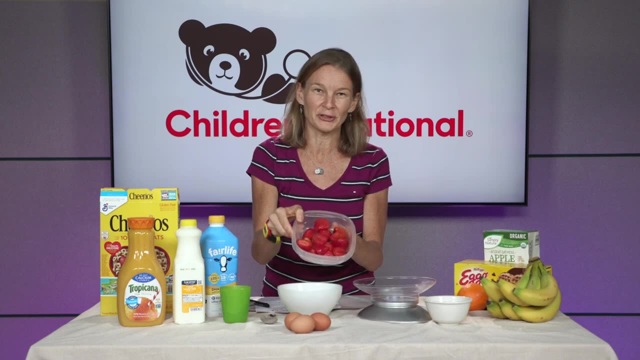 from fruit that also has carbs. The hard-boiled egg is a protein food. no carbs in that one one. so that's one thing I don't have to count. But the strawberries are a fruit and those have carbs as well. So basically the majority of the foods in my meal have carbs, and I'm 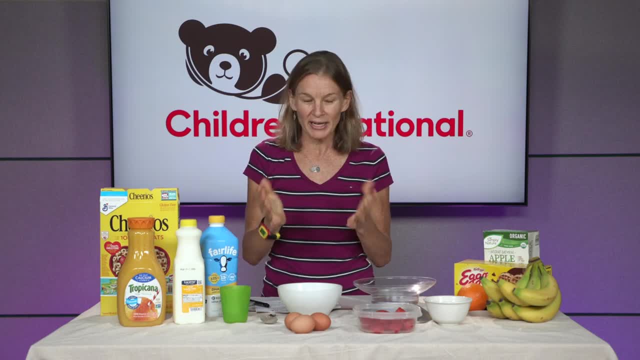 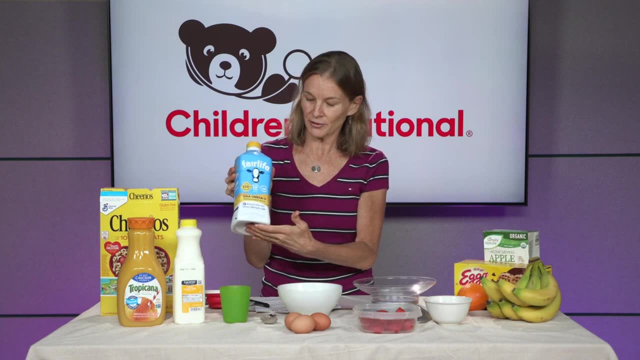 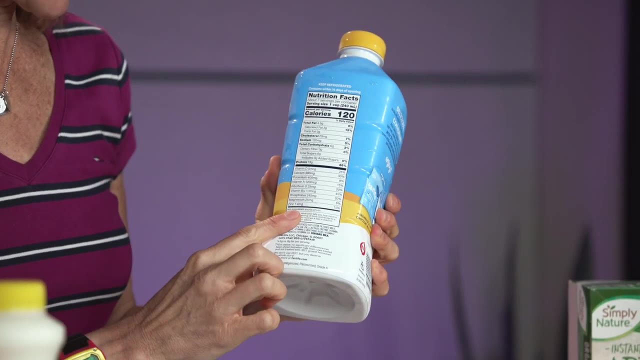 going to need to figure out how many. So when we're trying to figure those carbs out, there are three ways that we can do that. Many foods have food labels, So this milk, for example. this is a different brand of dairy milk called Fair Life. So this label has two things: that 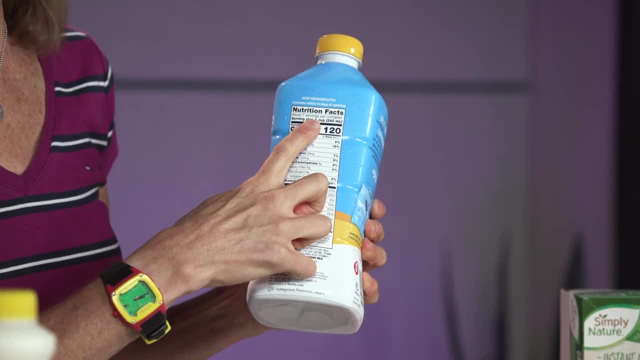 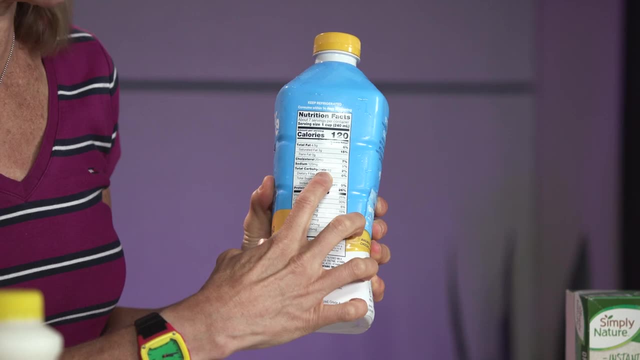 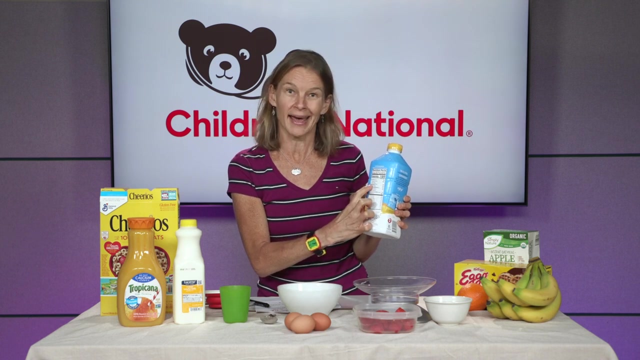 I want to keep my eyes on. One is the serving size, and for this it's one cup. So one cup of this milk has a total carbohydrate amount of six grams. So I need to know the serving size and I need to look at the total carbs. So if I have one cup of this milk, I'm going. 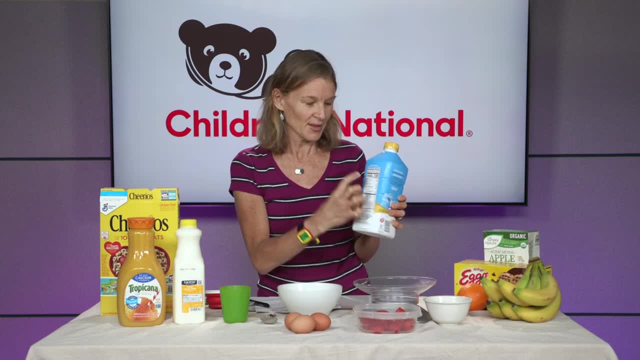 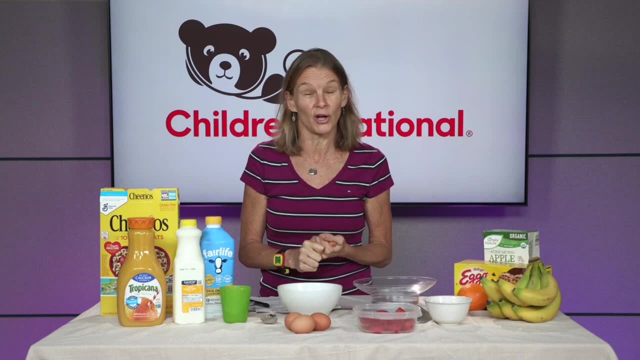 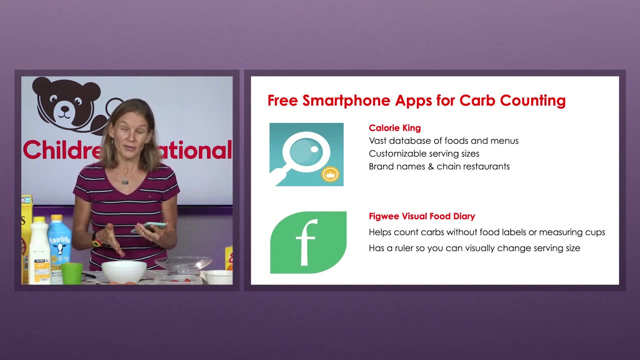 to add up six grams of carbohydrate for my carb count. All right, so that's one way looking at the food label. A second way is using an app or a book called Calorie King. I have a very handy app on my phone and I can look up any food out there, So this is helpful. 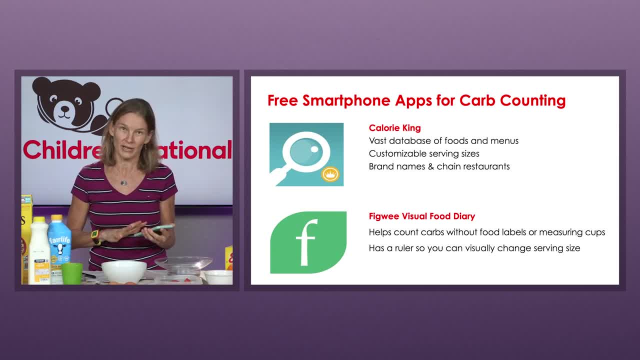 even if something does have a food label, I'm going to be able to find it in my Calorie King app. But Calorie King comes in really handy for fresh foods that don't have labels, like these strawberries. I don't know how many carbs are in these. There's no label. 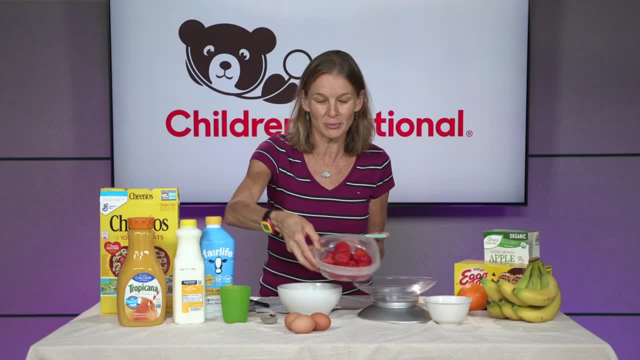 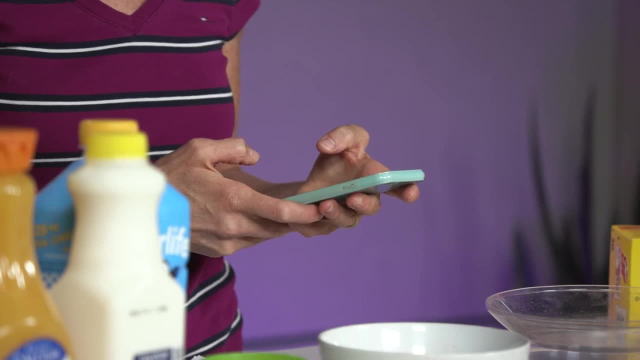 on them, and that's a good thing. It's good to have lots of foods that don't have labels. That means they're probably found in the produce section of the grocery store, So I can look up whole strawberries in my app. If I were to look that up now, I see that one cup of whole strawberries has 11 grams. 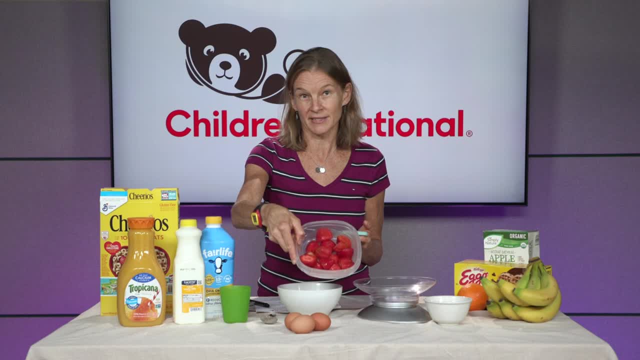 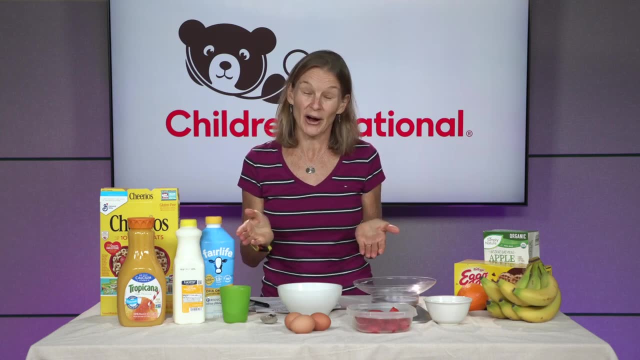 of carbohydrates. So I'm going to measure out one cup of these whole strawberries for my breakfast meal. All right, the third way to try to figure out carbs in a meal is to eyeball it, And this is not something we recommend, and I'm going to show you why. If I were to 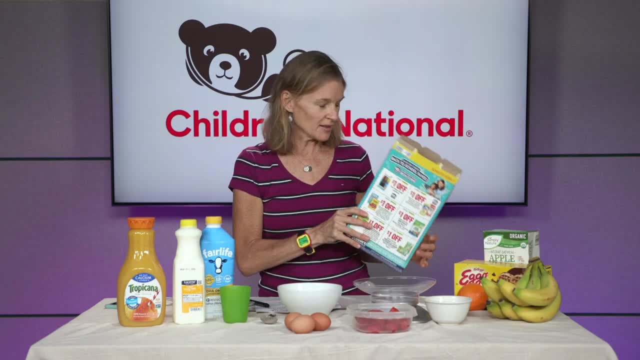 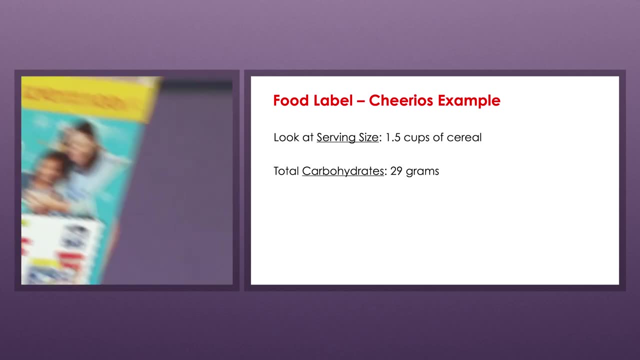 eyeball these Cheerios. now they say that on the label it says that one and a half cups of these Cheerios are one and a half grams of carbohydrates. So if I were to measure out, one cup of these Cheerios has 29 grams of carbohydrates. So I think I know what one. 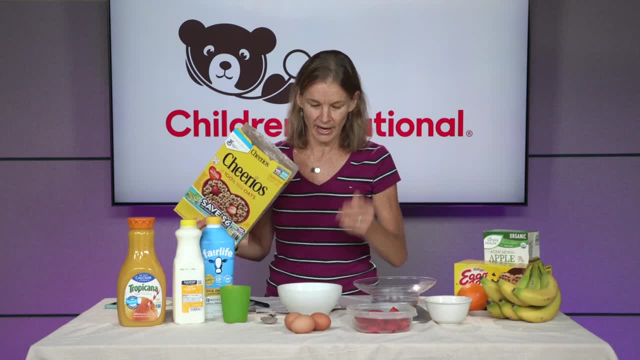 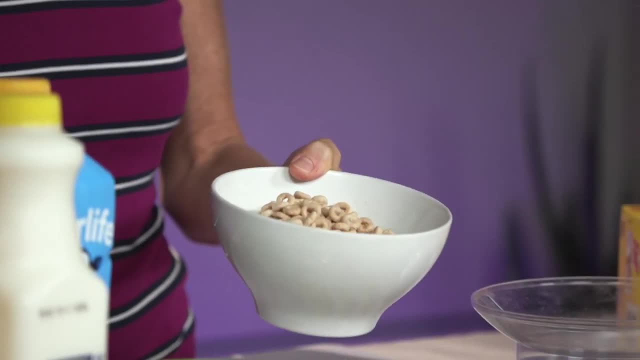 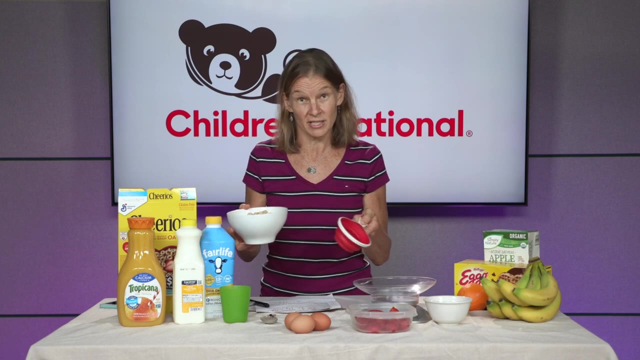 and a half cups looks like, So I'm going to actually pour that into this bowl. That looks about right to me. That's a good size bowl of cereal. one and a half cups, All right. so now let me go ahead and put that in my measuring cup and just see how close I was. 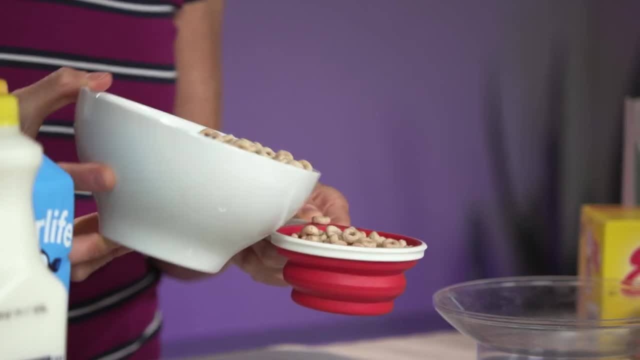 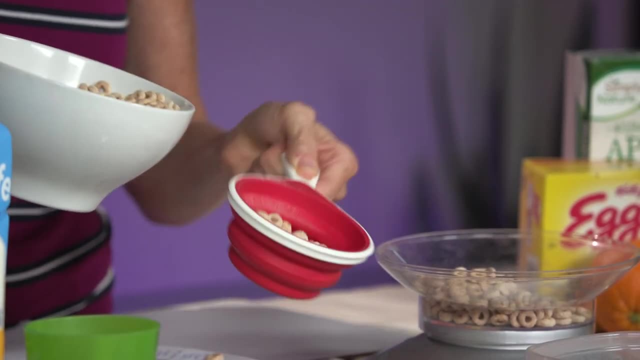 Hmm, Okay, that's one cup. I've already made a measurement. I'm going to go ahead and measure it. I've already made a mess and lost some of my Cheerios. Now I need about half of that one and a half cups. All right, that's one and a half cups. Look how poorly I estimated. 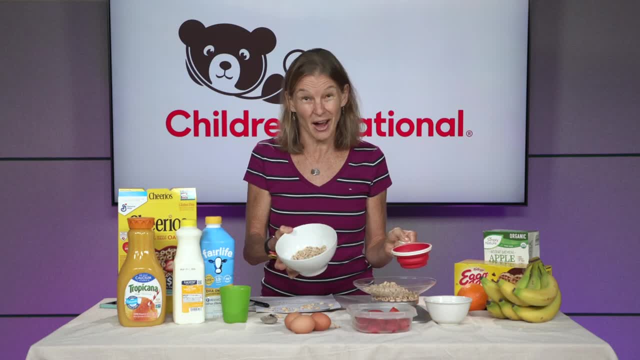 that amount of Cheerios. This is probably three cups worth of Cheerios, So eyeballing is not something we would recommend. in terms of carb counting your foods, Ideally you'll use your app, you'll use a book, the Calorie King book- or you use those food labels, All. 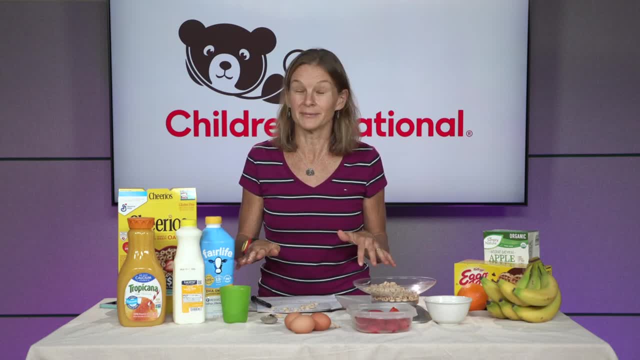 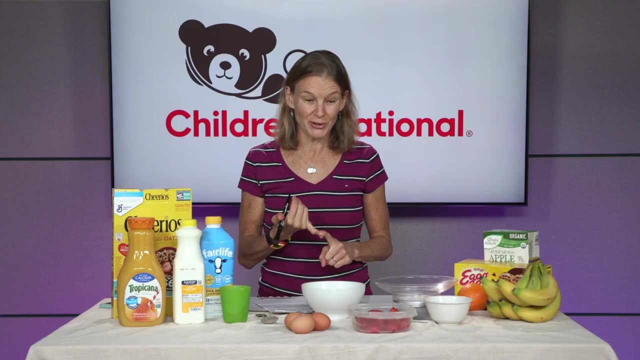 right Now, let me clean up this mess and we'll start our breakfast counts. All right, so let's count the carbs in our meal. We've got to count the carbs in the Cheerios. we've got to count the carbs in the milk, we've got to count the carbs in the orange juice and 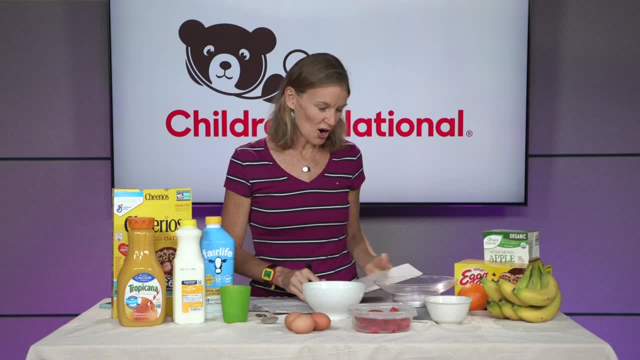 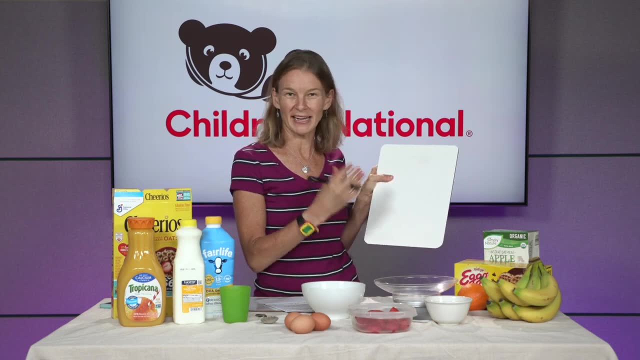 we've got to count the carbs in the strawberries, So that's four items. All right, so I'm going to start. I like having a whiteboard at home because I can just count every meal, wipe it down and have it ready for the next meal. All right, so my carbs. 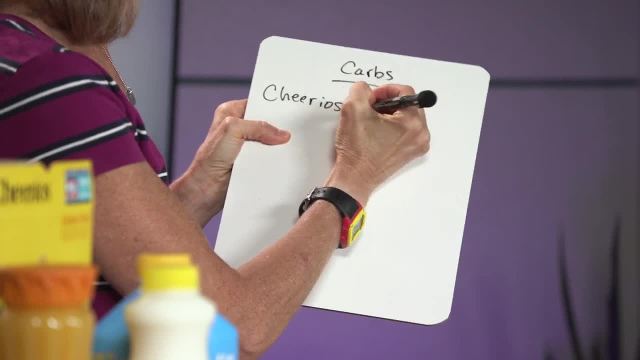 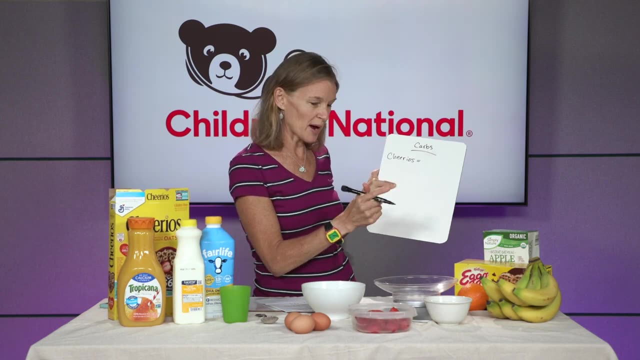 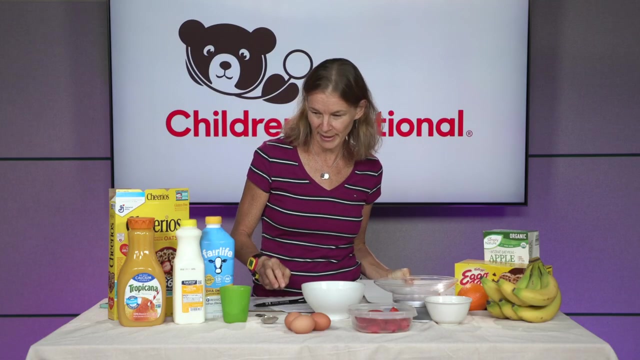 First off, we've got the Cheerios. So the Cheerios. the label said that one and a half cups was 29 grams of carbs. So I'm going to measure out one and a half cups and I'm going to write down 29 grams on my whiteboard. All right, Let's measure this out. So we've got. 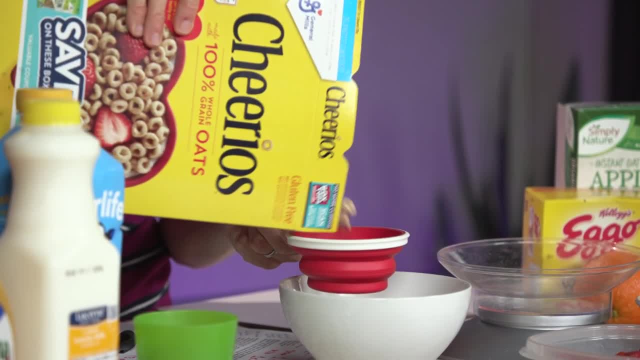 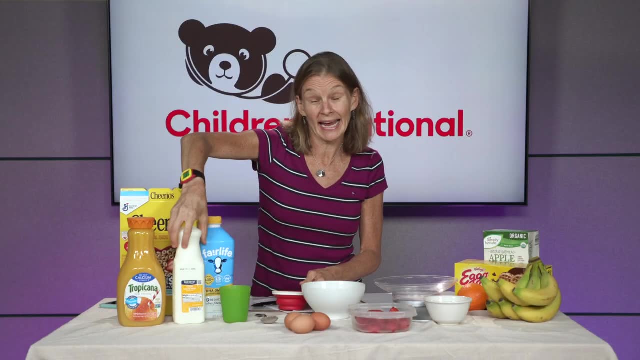 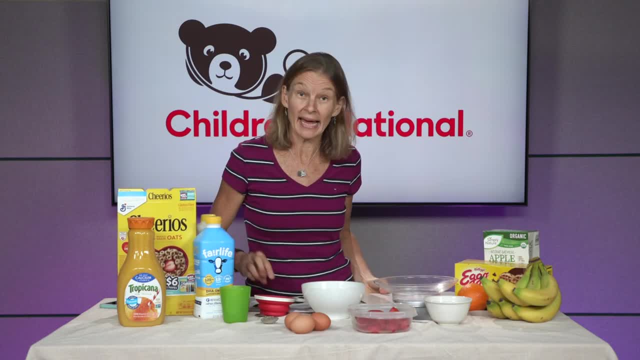 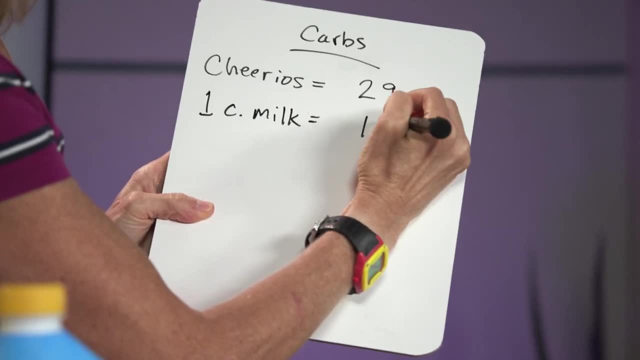 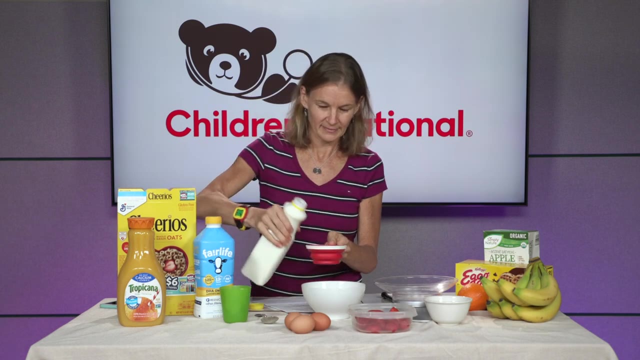 my one cup of milk, that's 13 grams of carbs. So let me add that to my list. So one cup of milk, 13 grams of carbs, All right. So we'll put that in. All right, you've got one. 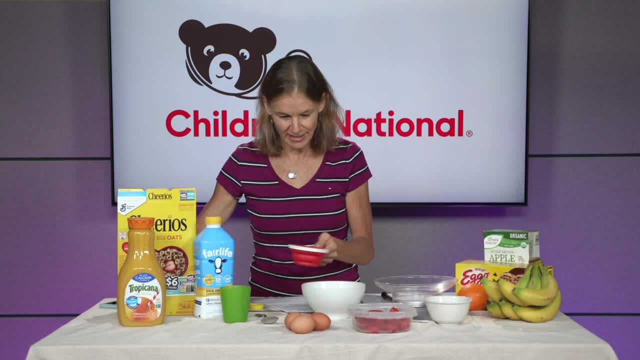 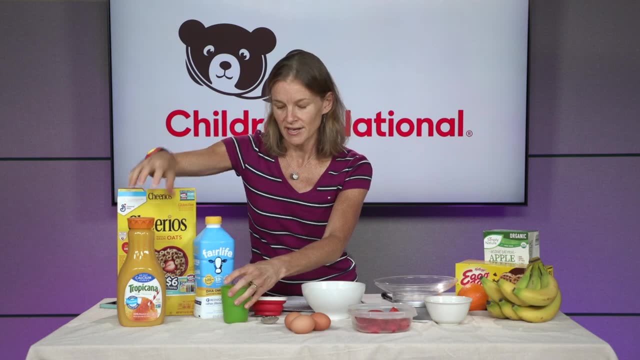 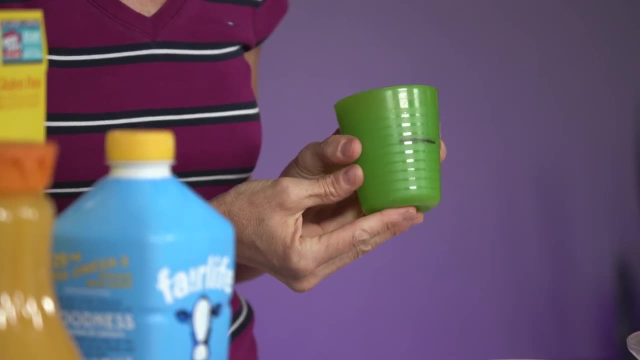 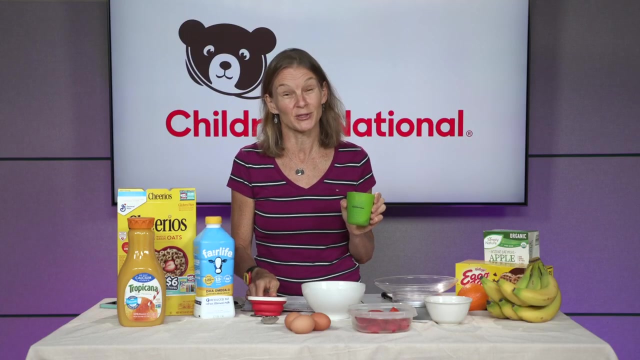 cup of milk Looks good, All right, Next up. Next up, I'm going to have a half cup of orange juice. So in my house we actually have two of our kids have type 1 diabetes. So one of our home hacks that we use is we've taken a bunch of our plastic cups and we've marked what one half cup is in Sharpie. So I don't have to use a measuring cup. I can just pour the orange juice up to this line and I know that's half of a cup. 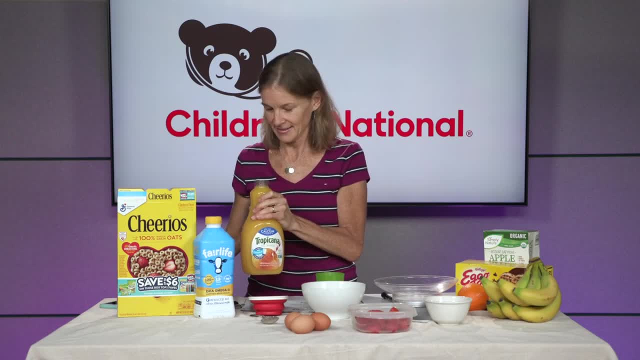 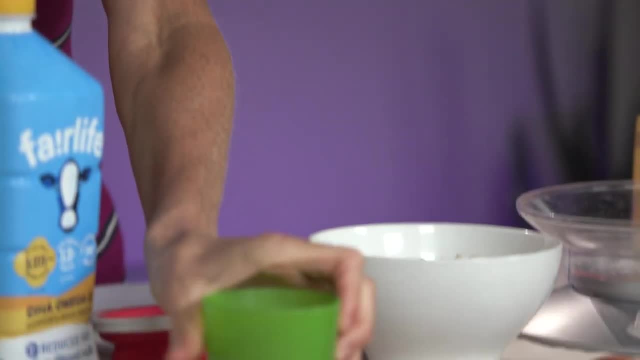 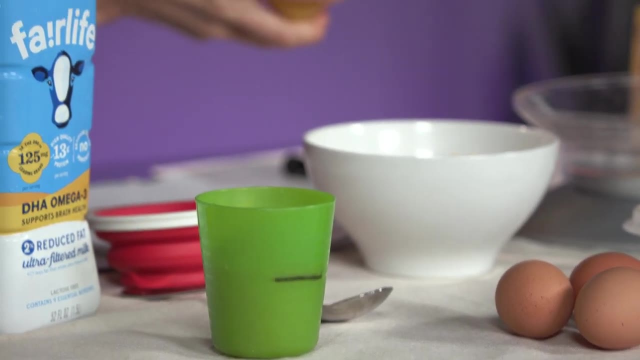 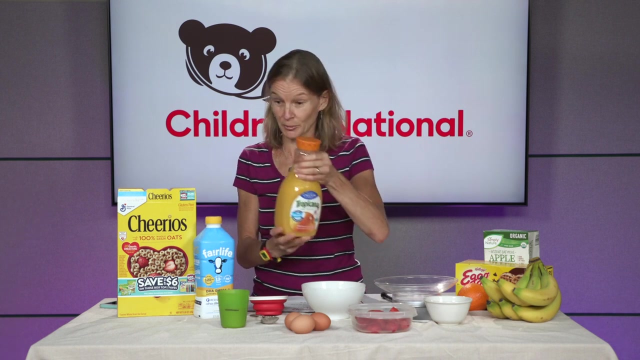 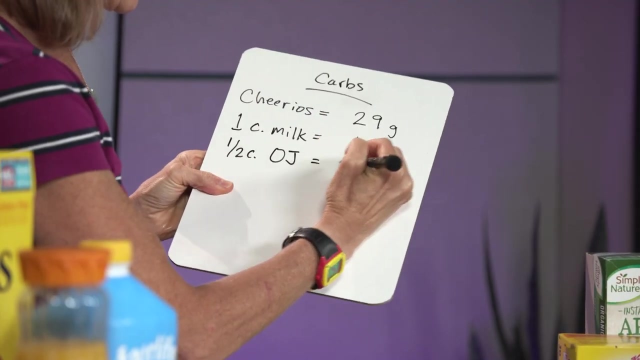 All right, There we go. We got our orange juice And a half a cup of this orange juice and I can tell from the food label: one cup is 26 grams of carbohydrates, So half of that would be half. a cup would be 13 grams of carbohydrates. So I'm going to write that down, All right. One half cup OJ- 13 grams. 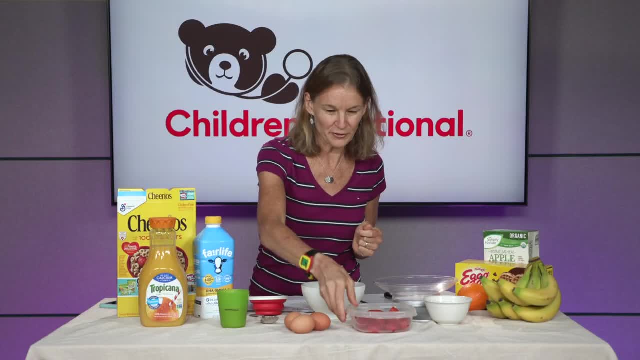 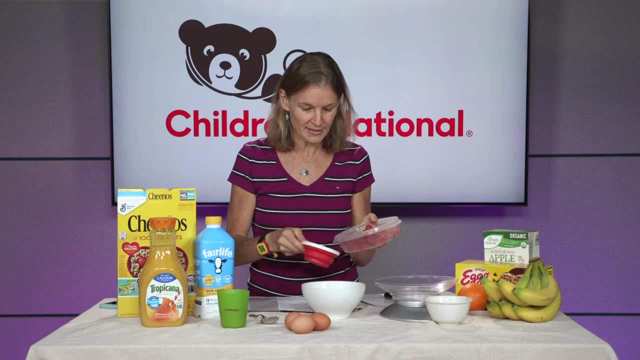 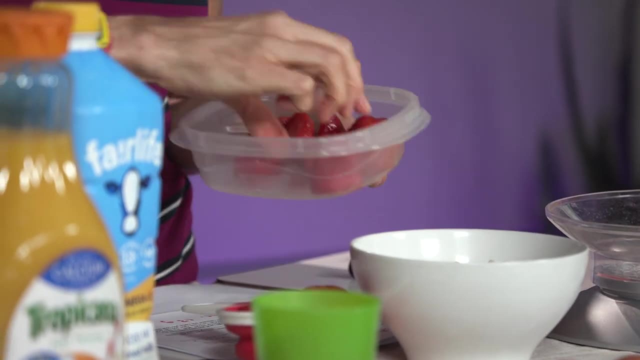 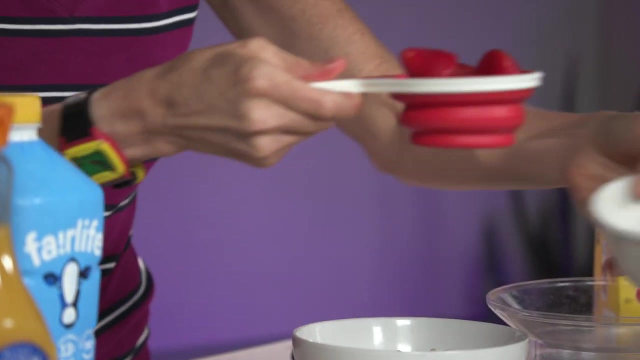 All right. Final thing: my favorite fruit, my strawberries. So I looked in my app and this was 11 grams of carbohydrates for a cup of whole strawberries. So let me just put some of these in my measuring cup. That looks about right, And I've got one cup of strawberries that I'm going to enjoy with my breakfast. 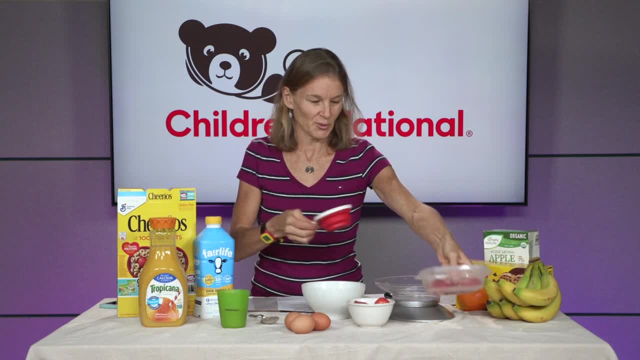 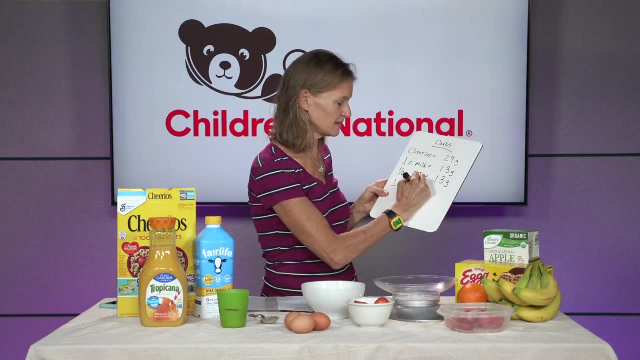 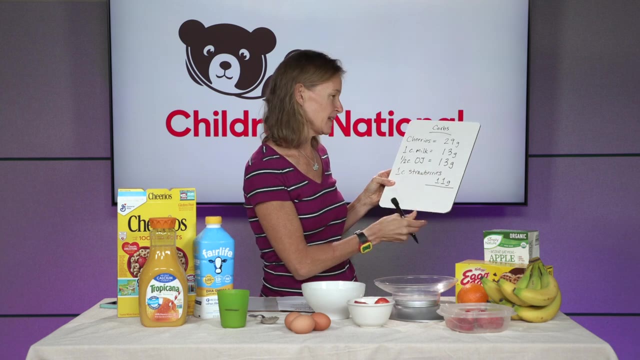 All right, So we'll add those to our list. One cup of strawberries is 11 grams of carbohydrate. Now, I might think I can do this in my head, but I'm not going to rely on my head for this addition. I'm going to use my calculator. 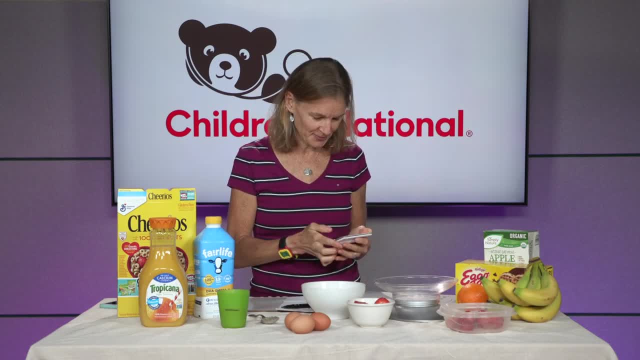 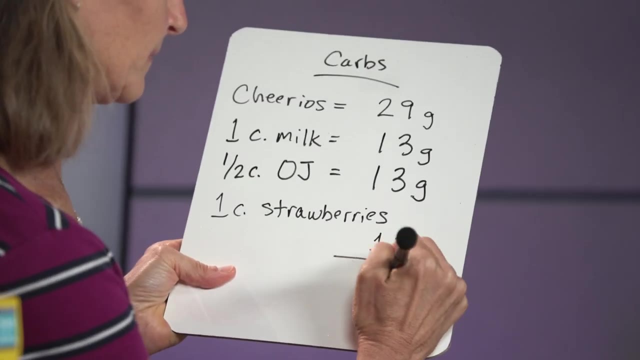 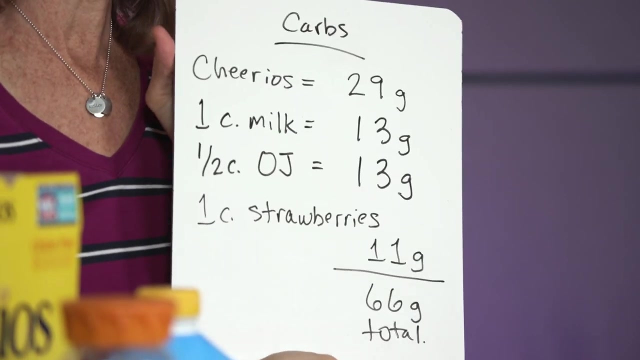 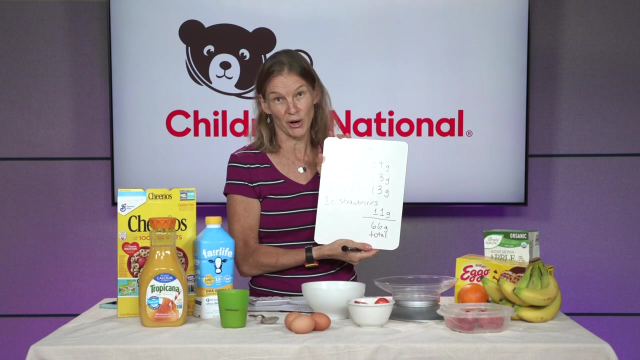 All right, We have 29 grams plus 13 grams plus 13 grams Plus 11.. I've got 66 grams of carbohydrates in this meal, All right. So now what I do with that 66 grams? the next step is you'll divide it by what your provider has given you as your carb ratio. 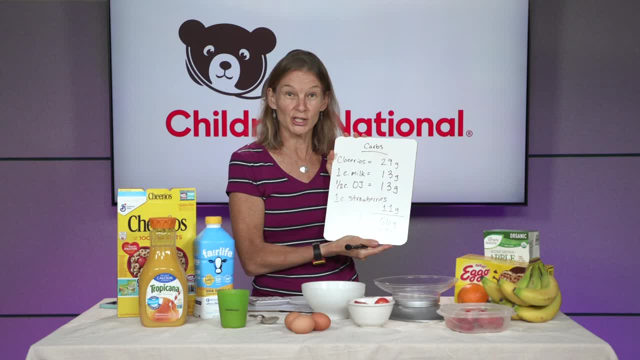 So I can give an example One of my kids at home. his carb ratio for breakfast is 20 grams, So he gets a unit of insulin for every 20 grams. So he wants to have a meal that's at this level and he had to understand that he wouldn't want to count his calories by 20 grams of carbohydrates. 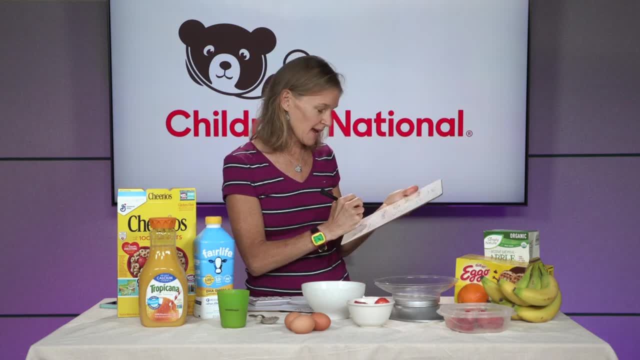 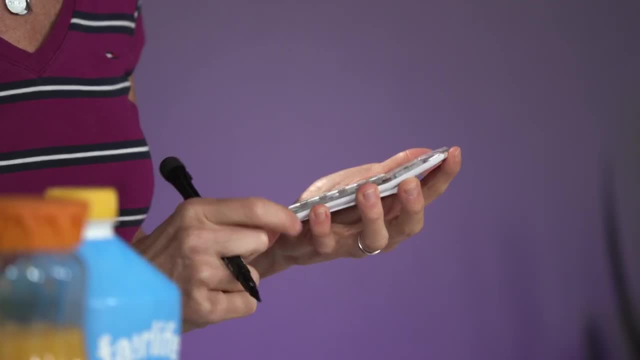 So I would take this 66 and divide it by 20. And then I would get my total insulin dose. So I'm going to use my calculator again: 66 divided by 20. 3.3 units of insulin for this meal. 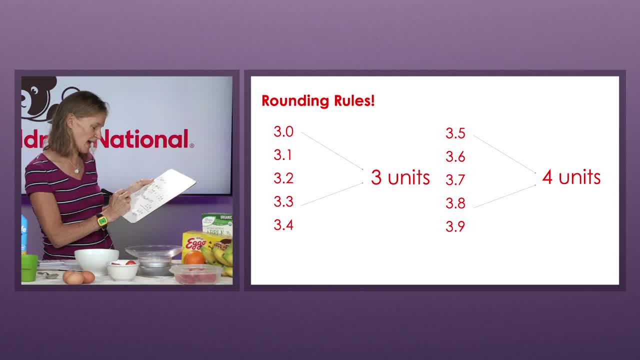 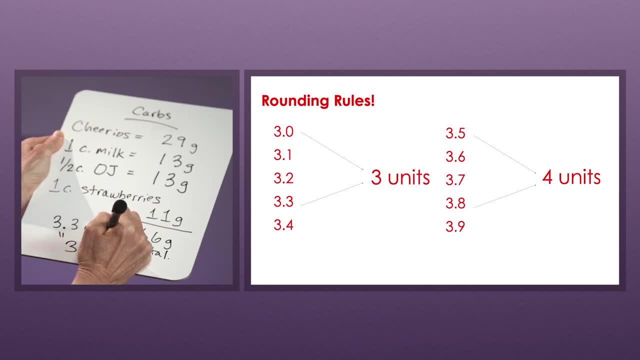 All right, And with his insulin pen I'm going to round that down to three units. So there we are All right. There we are All right. All right, All right. So what I'll do here. I've counted up my carbs. 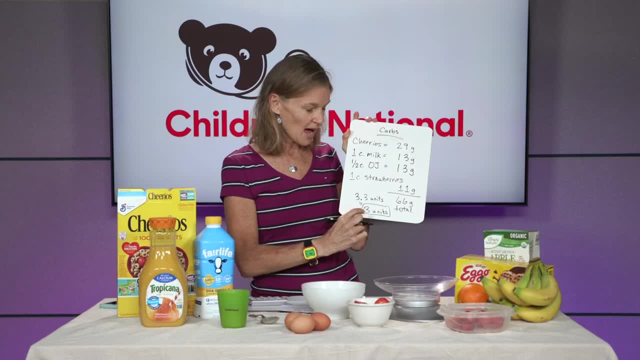 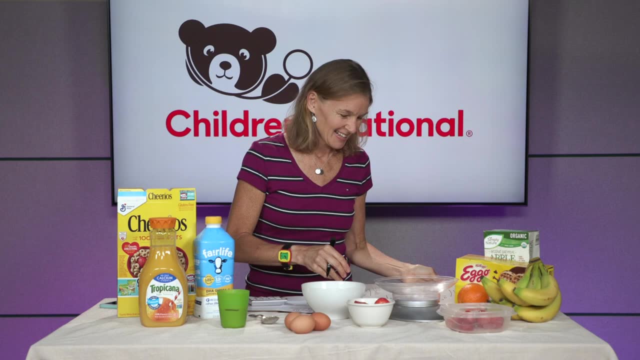 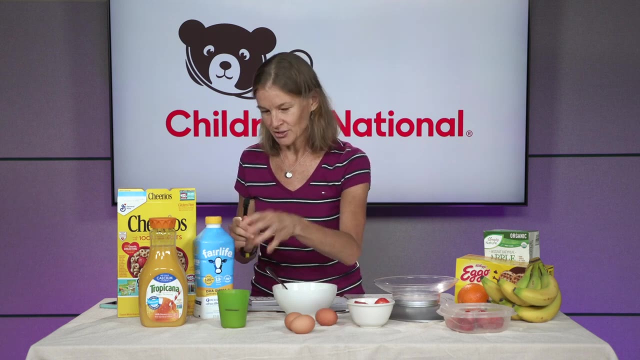 I've measured out my food, I've calculated my insulin. I'll take these three units of insulin and then I can finally eat, All right. Well, now what happens if I've eaten my bowl of cereal? I had my hard boiled egg. I drank my orange juice. 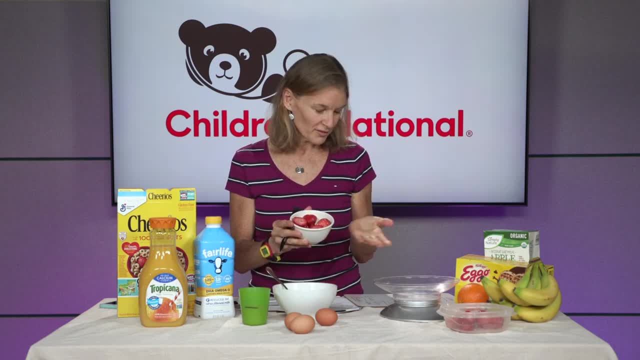 and I can't. I don't really have room for all these strawberries. Well, I've already taken insulin for all these strawberries, So I don't wanna go low from having too much insulin for the food that I've thought I was going to eat. 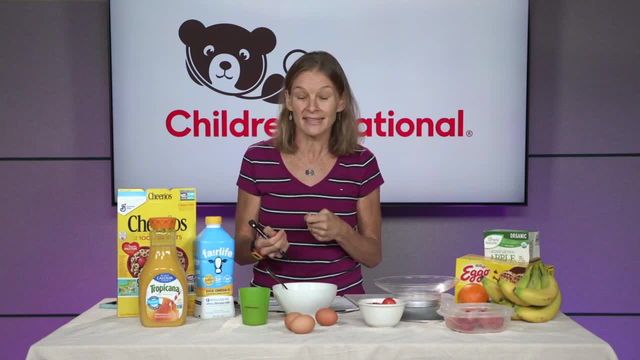 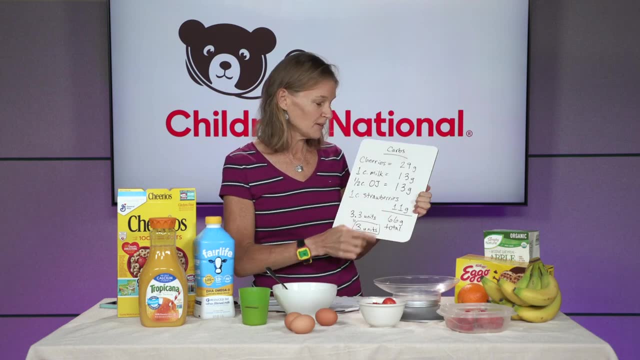 So what I can do is actually it's easier to drink carbohydrates than to eat them, So I can add a couple extra ounces of orange juice and make up for the half of the strawberries that I didn't have. All right, So say I need to make up five or six grams of carbohydrate. 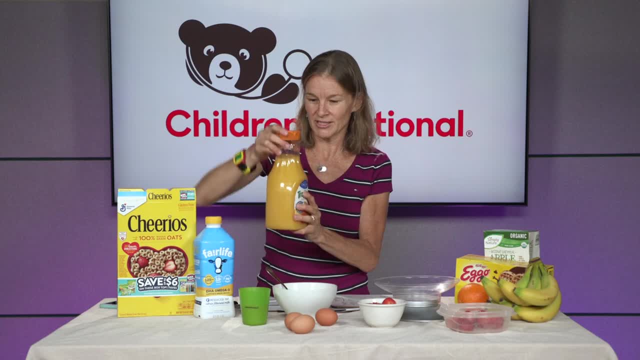 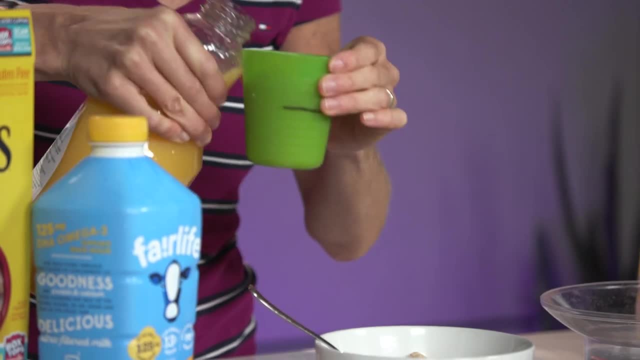 I can have another two ounces of orange juice, All right, So I could pour a little bit more in my orange juice cup in this case, All right, And you could measure that out: two ounces is a quarter of a cup, All right. and now that I've had all the carbs, 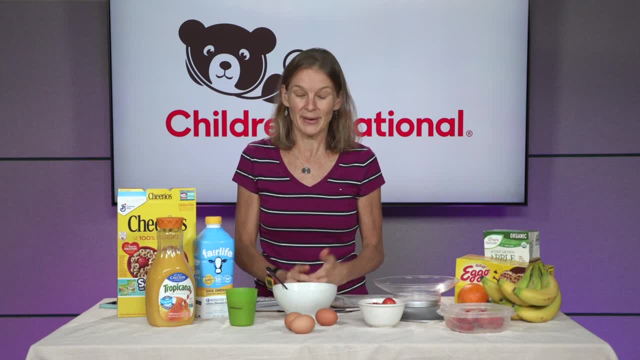 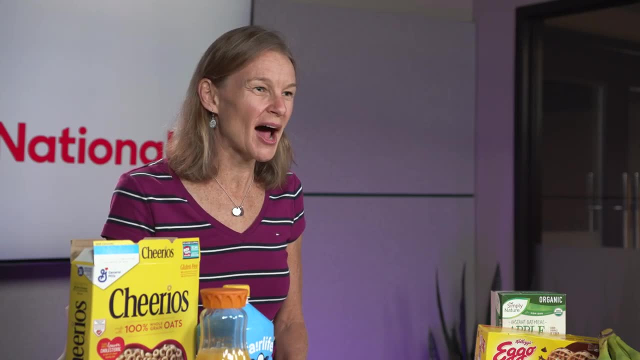 that I've given insulin, for I should be good to go And I've had my breakfast, I'm all filled up and energized and I'm gonna go outside and play. Okay, now let's review how we figure out how much insulin we're gonna give for this meal. 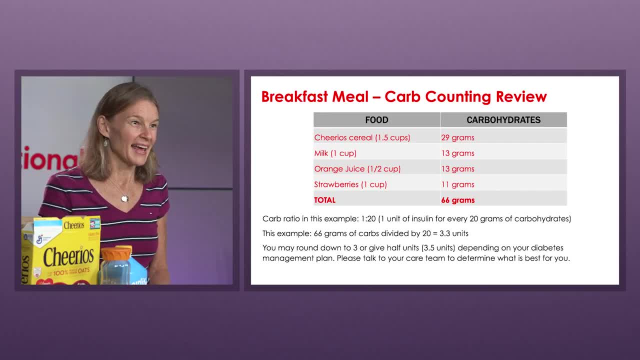 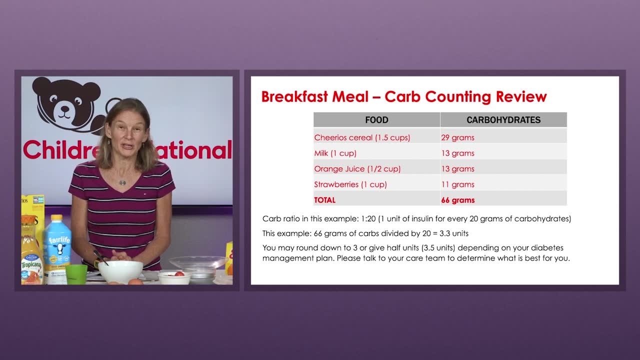 It had a total of 66 grams of carbohydrate, And what I do now is I divide that by my carb ratio that was given to me by my provider. In this example, I'm gonna use a carb ratio of one unit for every 20 grams of carbohydrates. 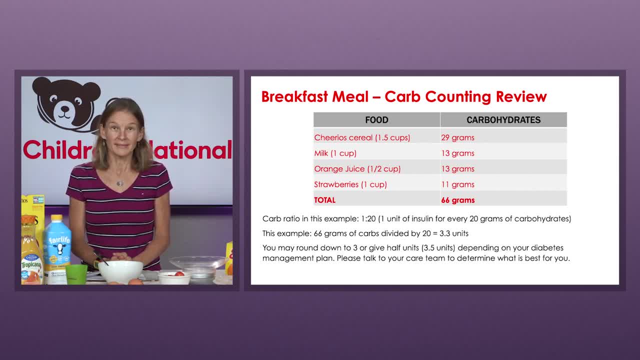 So I take the 66 grams and I divide it by 20. And on my calculator I get 3.3 units. If I'm using insulin by an injection with a pen, that means I round down to a whole unit of three units. 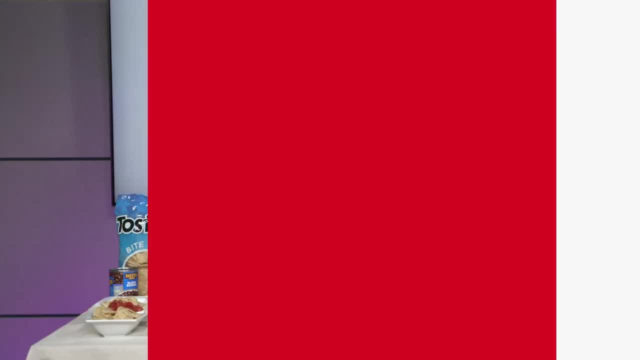 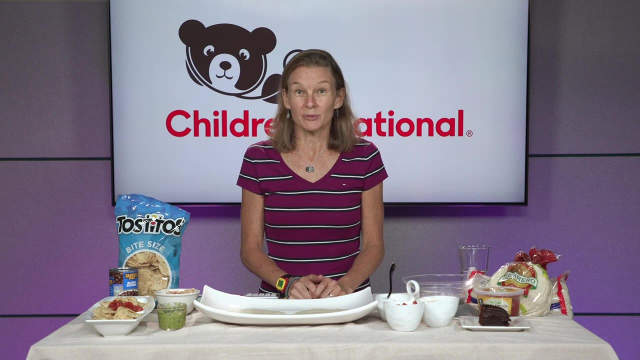 So in this case I would inject three units of insulin. All right, So let's make a dinner Tonight. for dinner we're gonna have some soft tacos, some chips and salsa and guac on the side, and then some homemade chocolate cake for dessert. 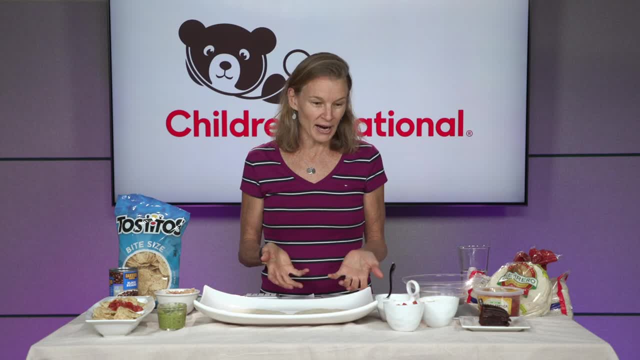 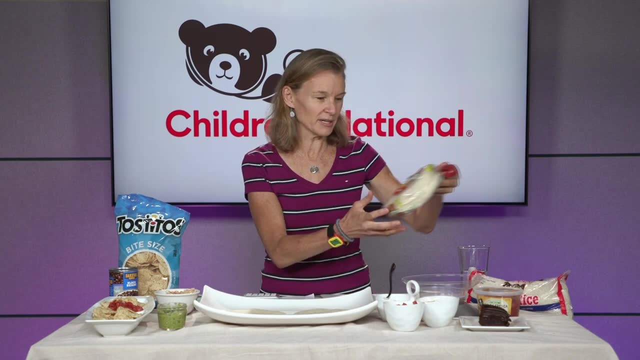 So first thing I need to do is figure out which foods have carbohydrates that I need to consider in my calculation. In this meal I'm gonna have tortillas, So this kind of brand of tortilla. They do have a food label, so I'll be able to tell the carbs from that package. 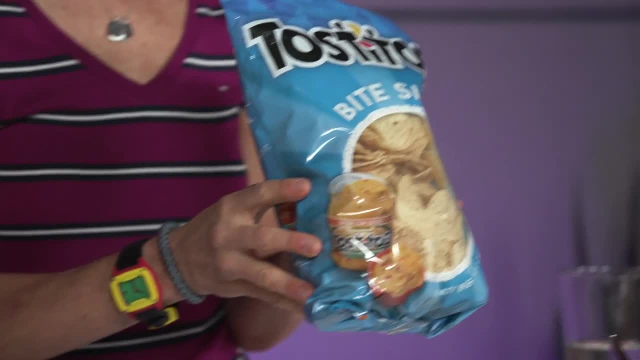 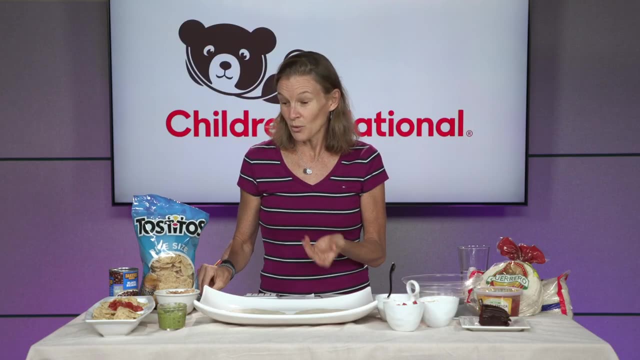 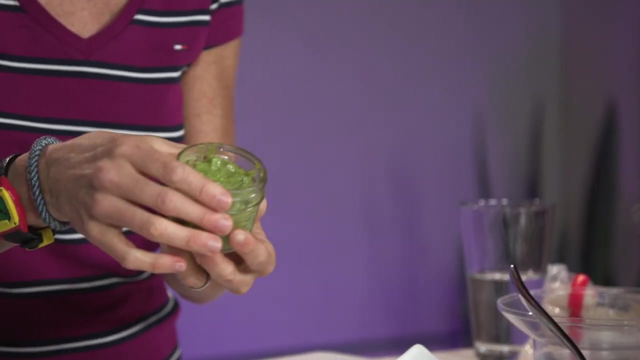 I'm also gonna have the chips which these also have a food label, So I can again tell the carbs in this food. The salsa and the guacamole are considered low carb foods. They're condiments, So I'm not gonna need to count the carbohydrates. 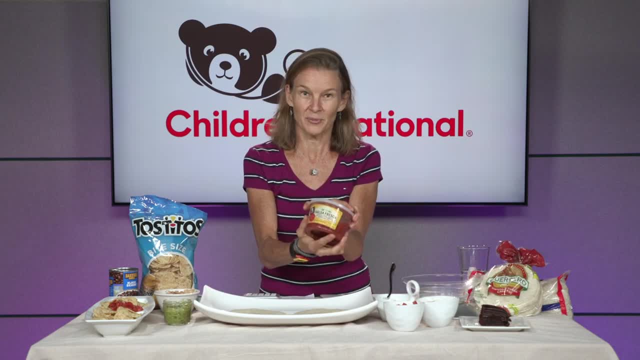 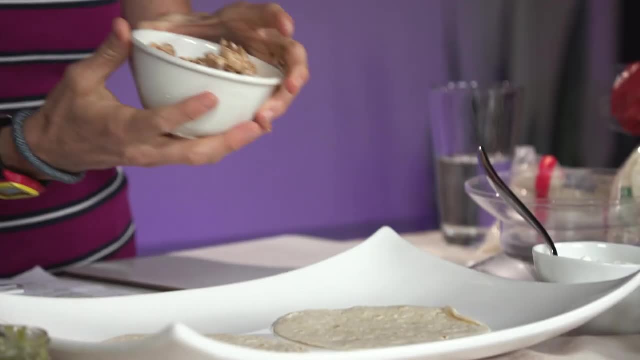 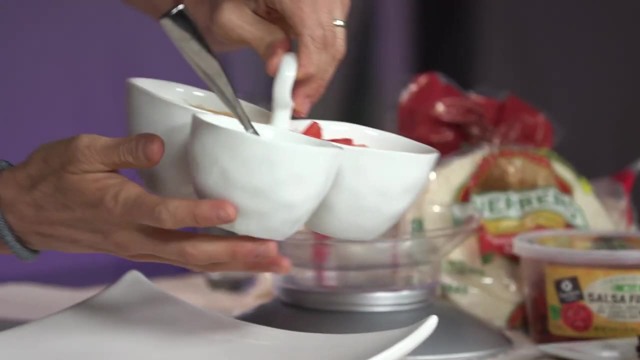 in those foods. This is a salsa fresca that we're gonna have with our dinner. Then I'm gonna fill the soft tacos with some chicken that I've cooked with just some spices, Some fresh tomatoes chopped up, some cheese and some sour cream. 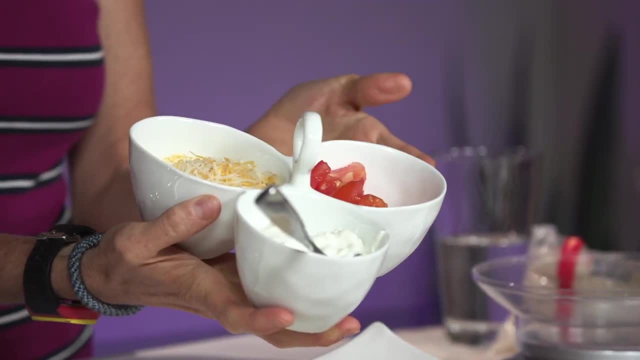 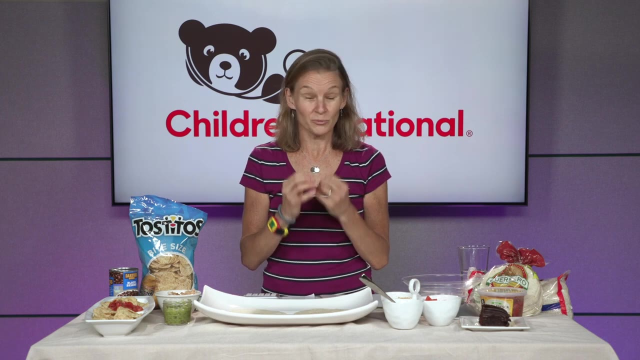 So all these items are very, very low carbs, So I'm not gonna need to consider those in my calculations. And then, even though I might not have dessert with my dinner, I know I'm gonna have it pretty soon after, So I can add those carbs from the dessert. 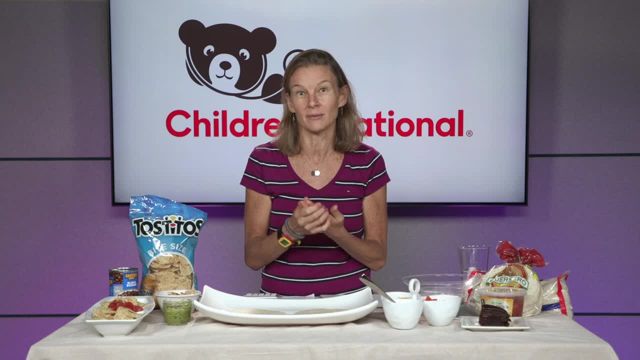 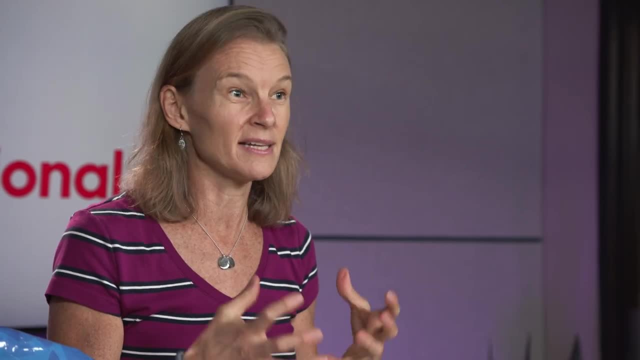 in my total calculation and give all of that insulin at the beginning of the meal. As long as I don't wait too long to have dessert after it's fine to group all of those carbs into that one insulin dose and give that at the beginning of the meal. 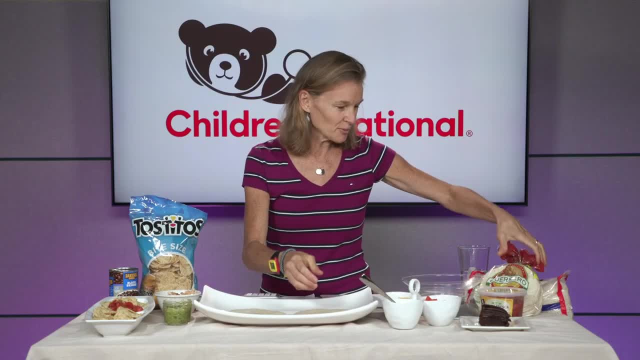 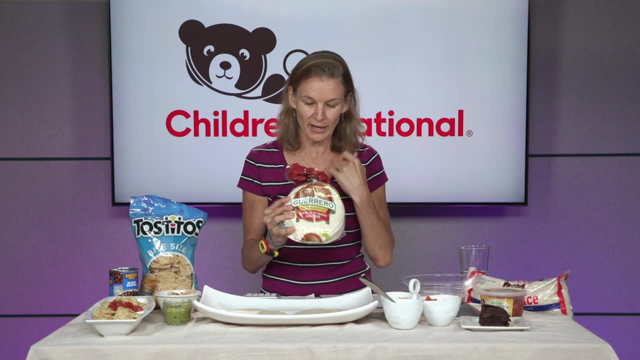 All right, so let's make our meal. All right, so I'm gonna have- I think I'm gonna have- two small soft tacos. So each one of these tortillas has 15 grams of carbohydrate. So in my two, that means I'm gonna have 30 grams of carbohydrate. 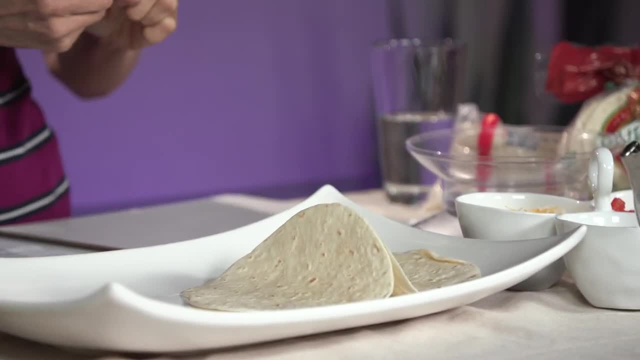 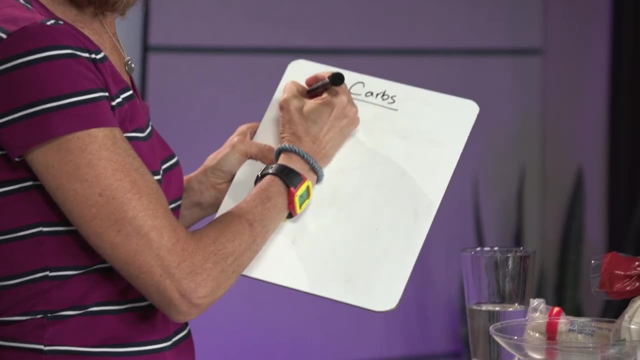 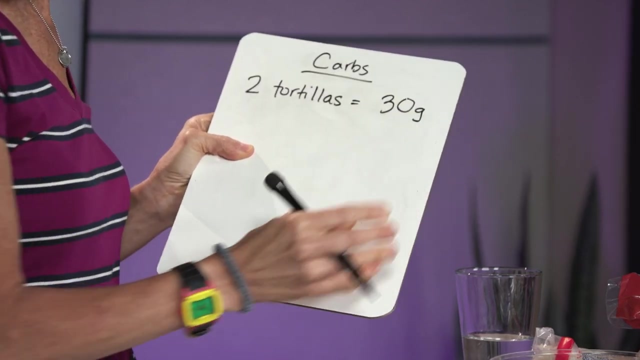 So we're gonna start by building those and I'm gonna use my whiteboard again. All right, I'm gonna write down my carbs. So two tortillas, 30 grams of carbs, All right, so I have those two tortillas. 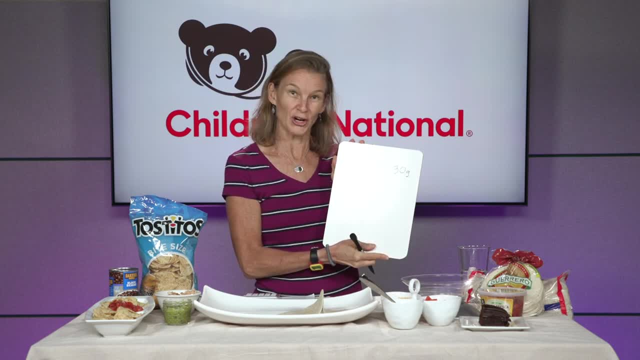 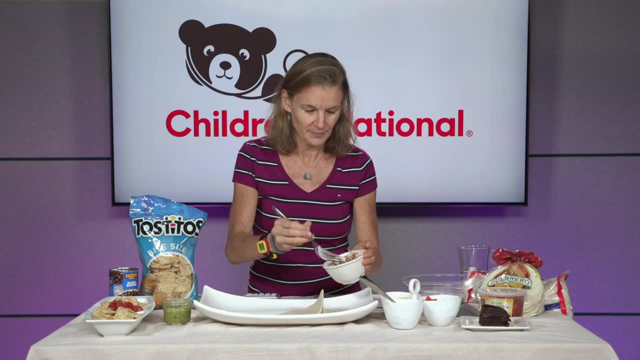 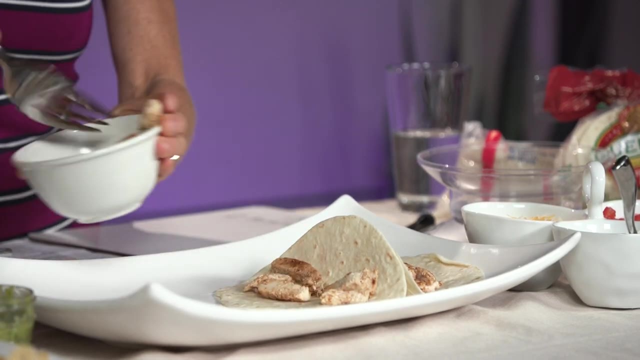 Pretty sure that's what I'm gonna wanna eat. I'm not gonna be hungry after 30 grams of carbohydrates. All right, now I'm gonna fill those tortillas with a little bit of chicken. All right, I'm gonna add a little bit of sour cream. 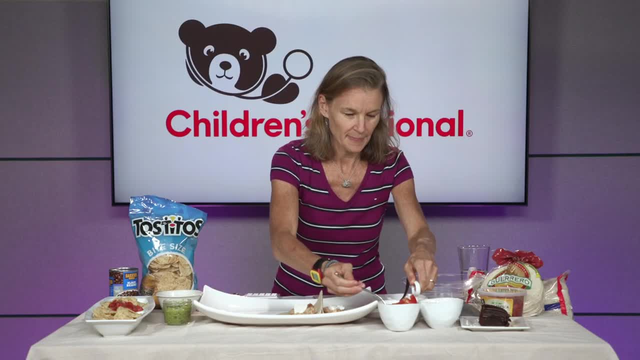 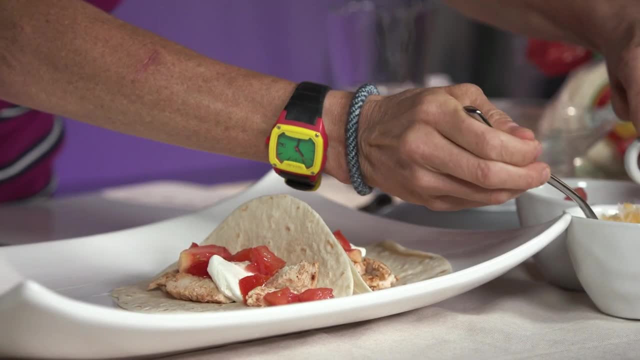 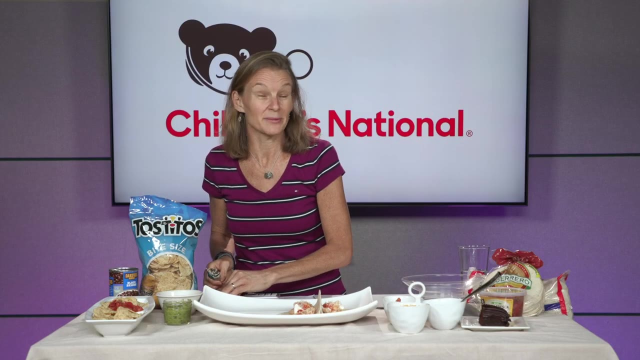 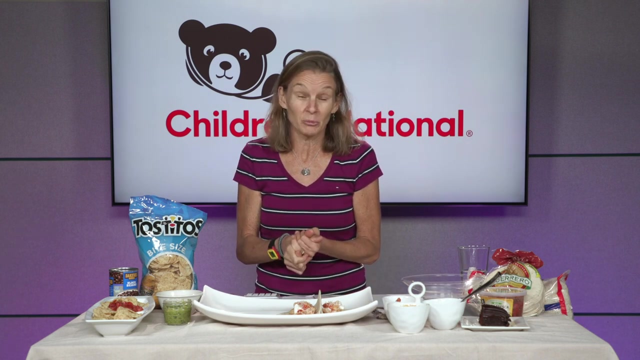 I'm gonna put on some fresh tomatoes And then also a little bit of shredded cheese. All right now, you can heat those up. You can eat them as is, however you prefer. All right now. in addition to these tacos, I'd like some chips and guacamole and some salsa. 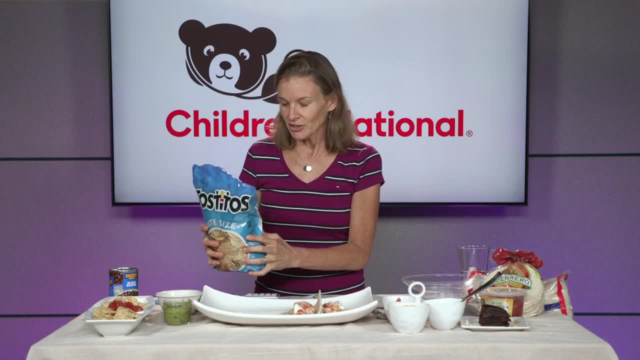 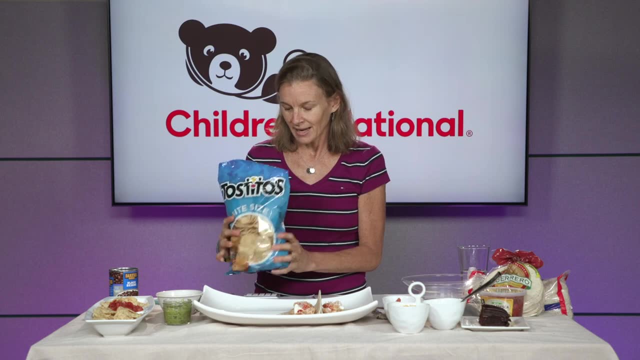 So I do need to count the carbohydrates in the chips. Looking at the label, these have. it says 24 chips is about 18 grams of carbohydrate. I'm not sure I really feel like counting out 24 chips, and a lot of them are broken. 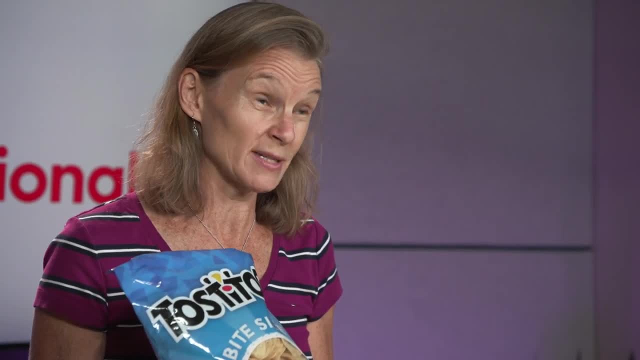 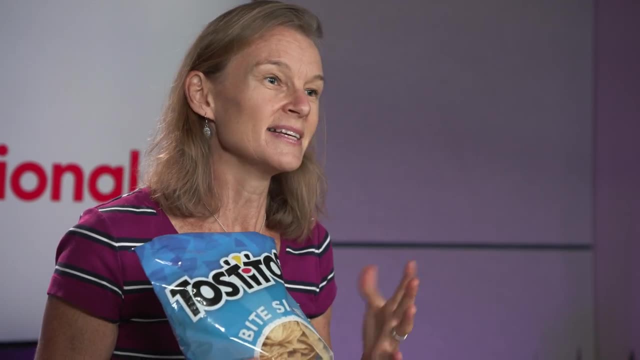 So for this calculation, what I'm gonna do is use my food scale. You don't have to have a food scale. You don't have to have a food scale to count carbs, but I do find it really handy to have one for certain things like snack foods. 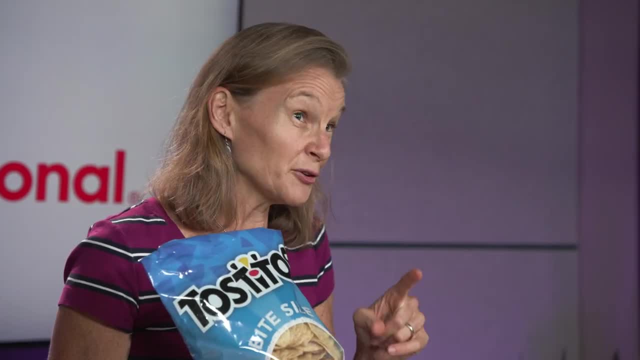 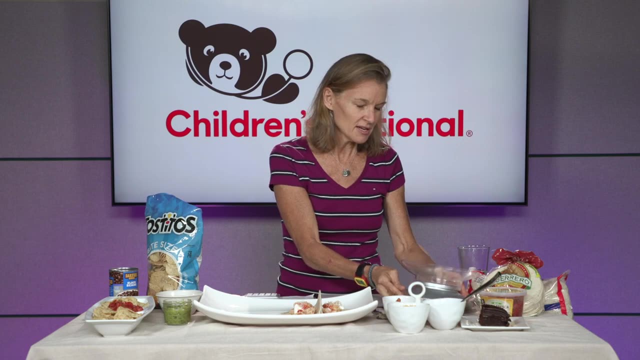 sometimes breakfast cereal, So dried fruit actually is another one I like to use that for. So on my food scale I have this here. I first just need to zero it out. This one has a bowl that comes with it, which is nice, because then you could even just 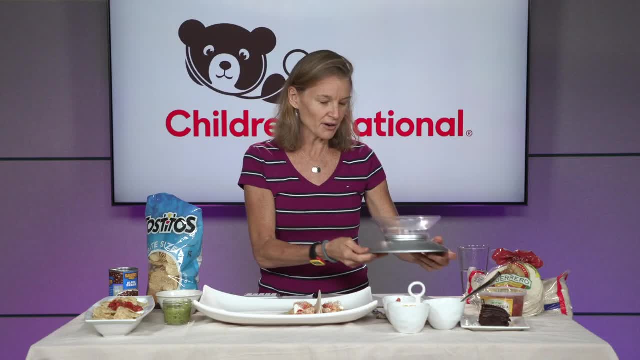 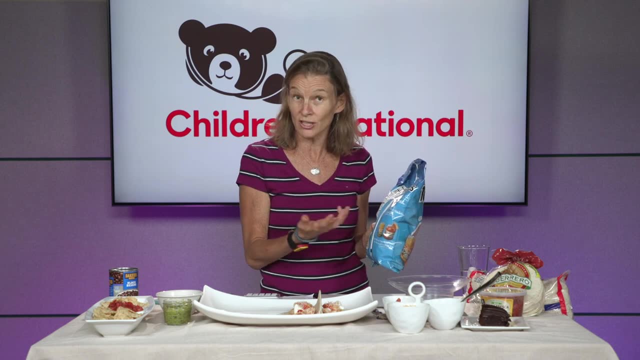 put your chips in this bowl and take it to the table and have that. But I'll first zero that out And in looking at the food label I see that the 24 chips weigh 28 grams. So I'm gonna just pour out until I get to the 28 grams. 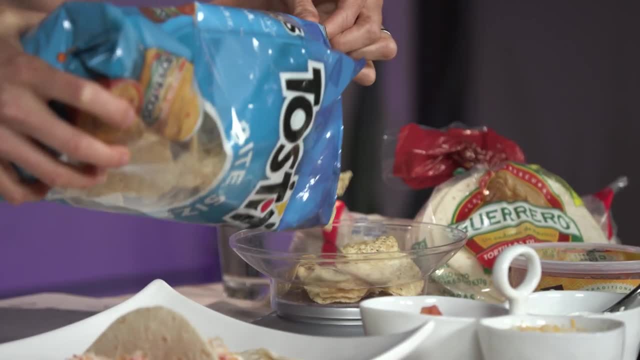 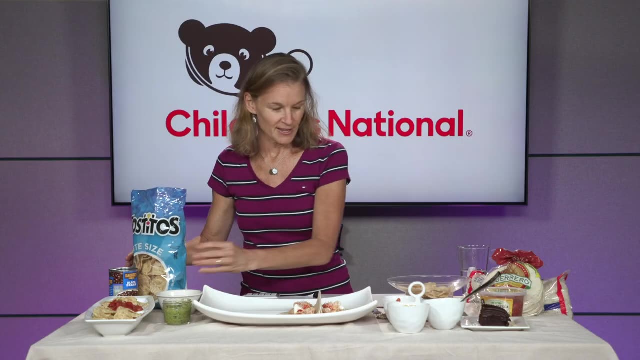 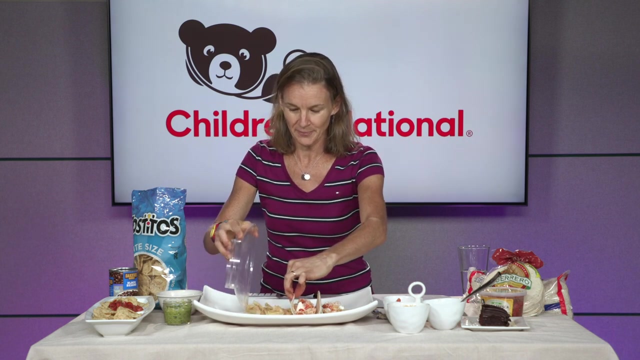 on my food scale. All right, it's got 33, so I'll put a couple back, All right. So to me that's a lot easier than counting out 24 chips. So I have my chips here, Put them on my plate and I'm gonna write that down. 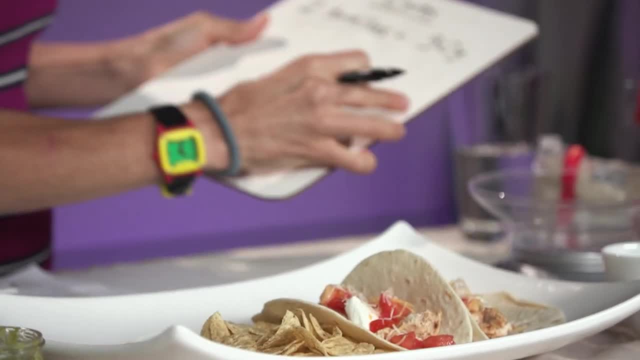 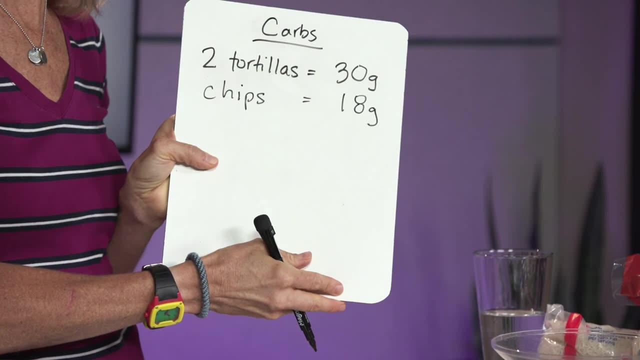 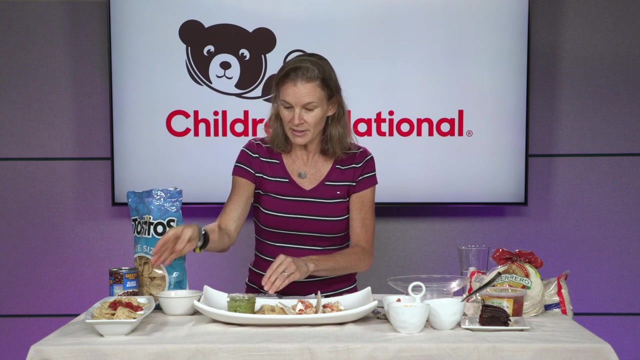 on my whiteboard. So the carbohydrates? there were 18 grams, All right. so my chips: 18 grams of carbohydrate, All right. Now I have my condiments, which I'm not gonna need anything counted for. So I have my salsa and my guacamole. 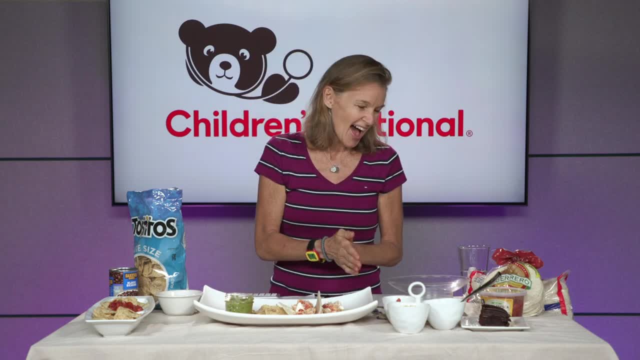 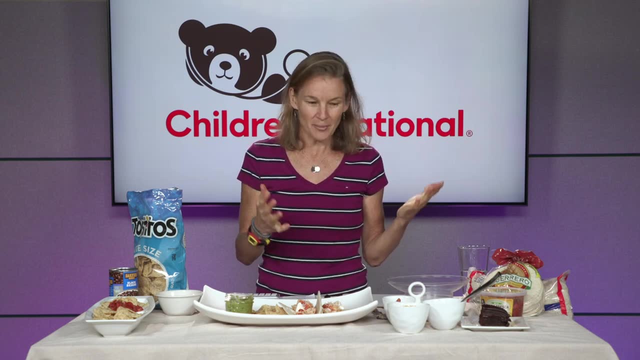 So I can just actually have as much of those condiments as I want. Now I wanna add the calculation for the chocolate cake with the frosting This came from. This came from a homemade recipe, so I don't have a carb count. 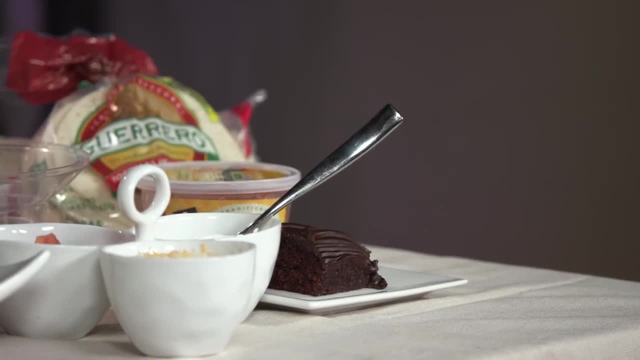 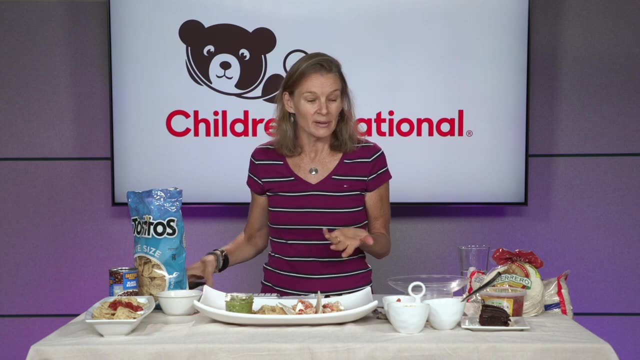 I think the you know when ingredients are eyeballed and nothing is specifically measured. you do have to. you have to do a little bit of guesswork, But I can use my app and I can look in Calorie King to see what an average size piece of chocolate cake. 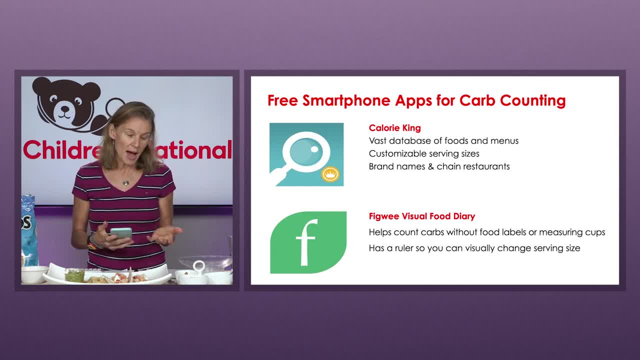 with frosting would count for carbs. Another app you can use is called FigWee And with that you can actually take a picture of the food and it will show you the amount of calories that you have. It will show you the size on the plate. 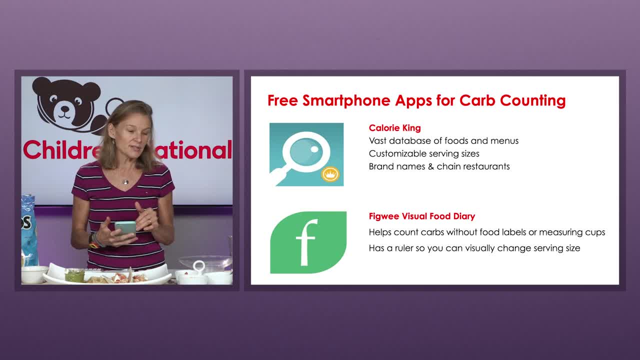 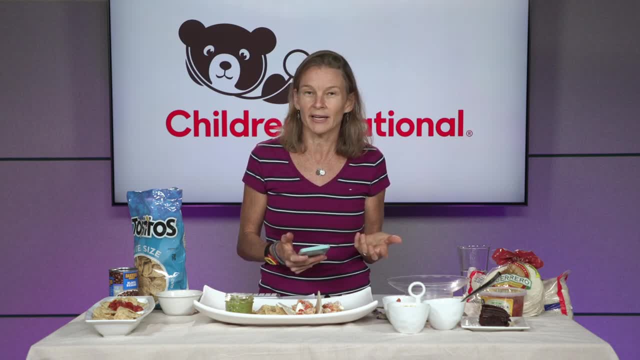 and give you an estimated carb count. And also if you're on an insulin pump. the insulin pumps sometimes have food libraries where you can look up food items. So if you don't have Calorie King or you wanna try another app, there are some other options out there for you. 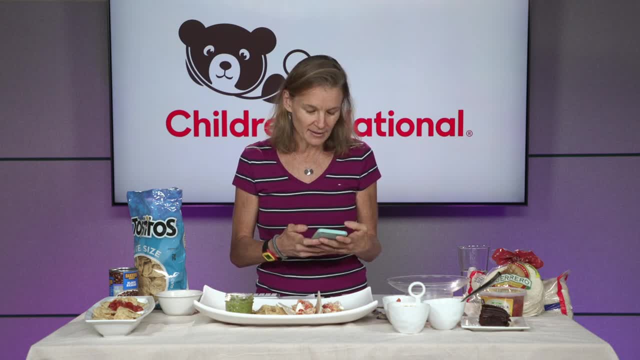 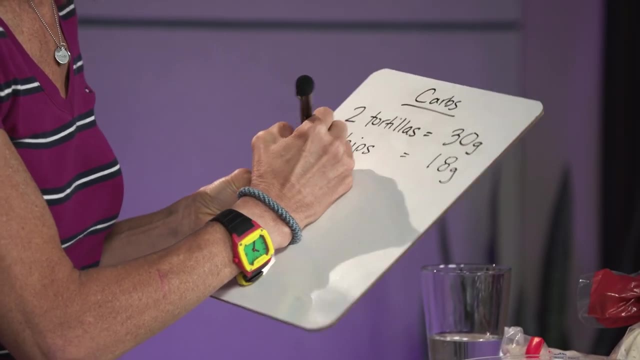 So looking in my app it looks like a commercial brand. chocolate cake with frosting with this size is about 42 grams of carbohydrate, So I'll just. I might not be exactly right, but I think that's pretty close. So my cake. I'm gonna write that down as well. 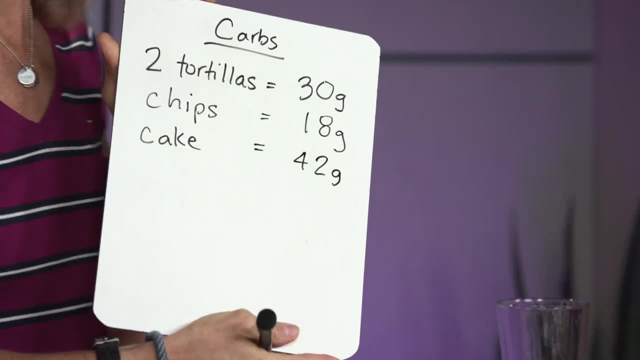 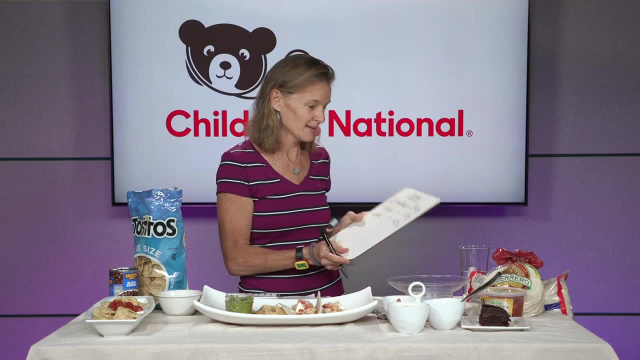 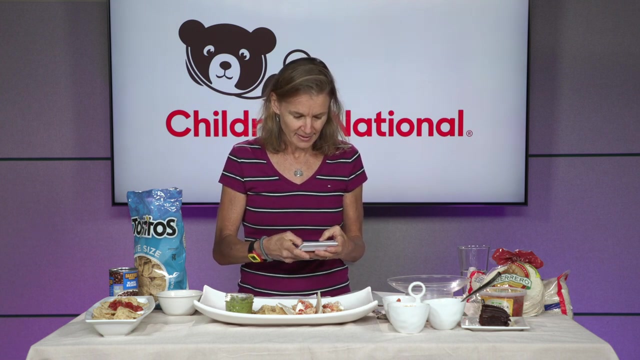 42 grams of carbohydrate. All right, so what I'm gonna do is add that up, I'm gonna divide again by my carb ratio and figure out how much insulin I need for this meal. Okay, pulling out my calculator, We have 30 grams, plus 18 grams in the chocolate cake. 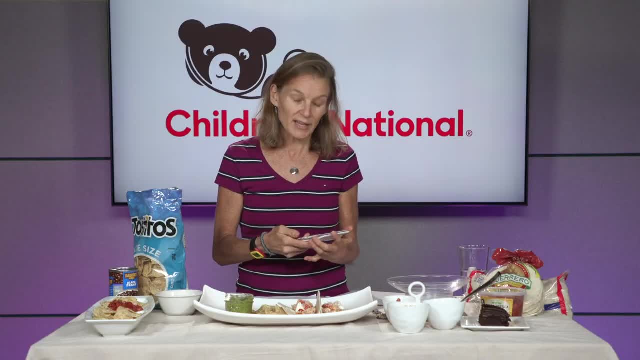 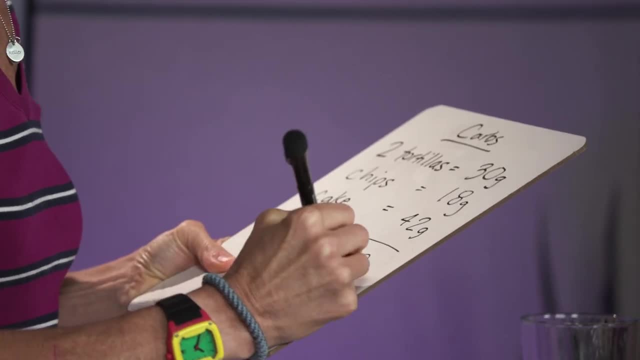 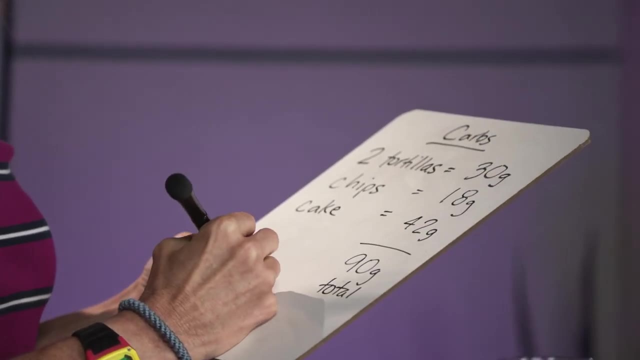 So that's all the chips and 42 for the cake. So that's a total of 90 grams of carbohydrate. Okay, 90 grams total for this meal. I'm gonna take that. I'm gonna divide that by my carb ratio. 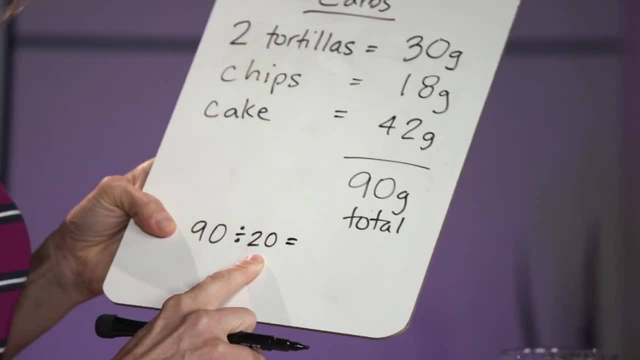 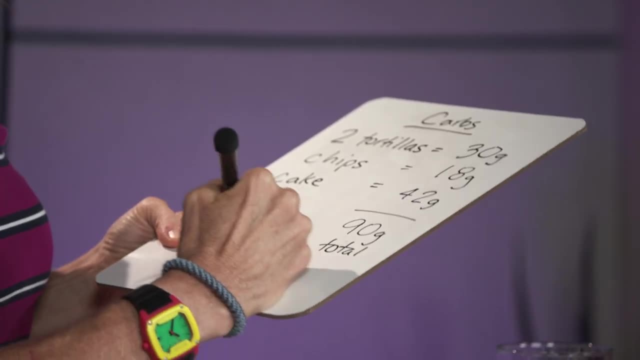 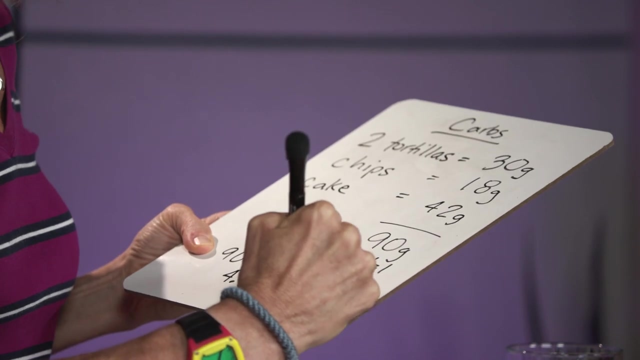 which was given to me by my provider, And that's 21 units for every 20 grams of carbohydrate And that comes out to 4.5 units of insulin, And that one I'm gonna round up to five units With our basic rounding rules. 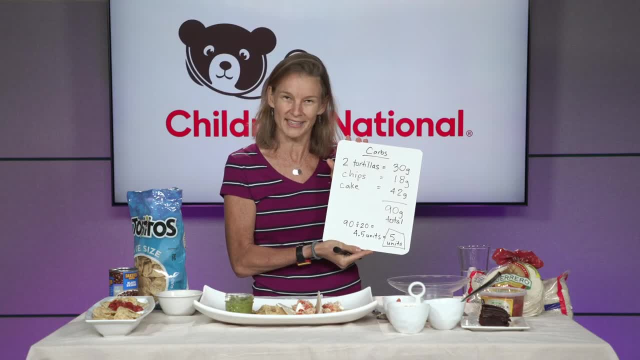 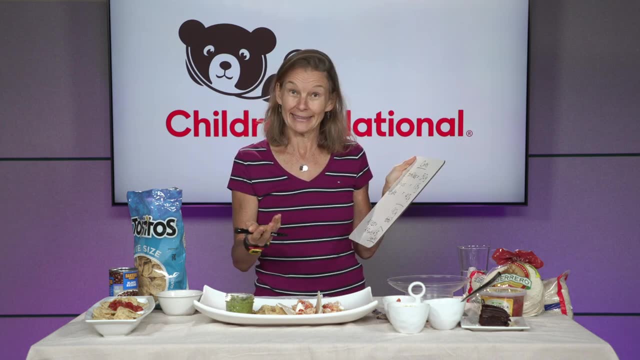 if it's 0.5 or more, you round up. If it's 0.4 or less, you round down. So I'm gonna inject five units of insulin for this meal, and then I'll be able to eat it. All right, start over again. 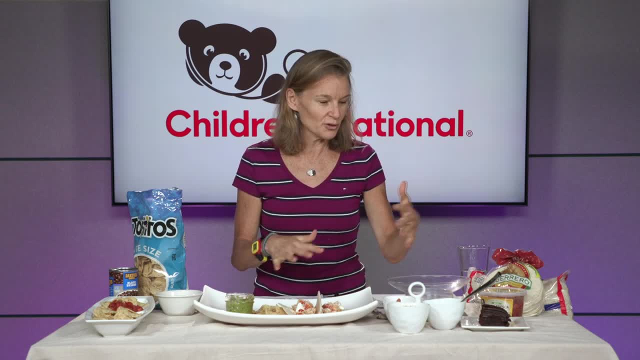 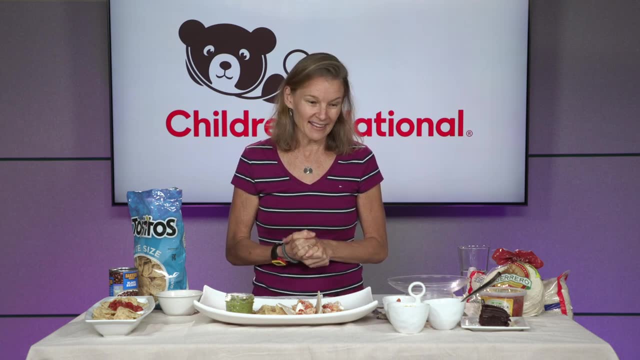 Okay, now let's say I've eaten all this food- Maybe I even already ate my chocolate cake- and I'm still hungry. What do we do? We've already taken our insulin, and that insulin was simply for these carbs. Well, don't forget that, you can still have. 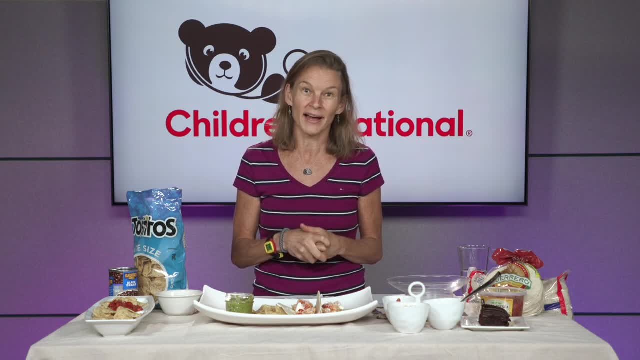 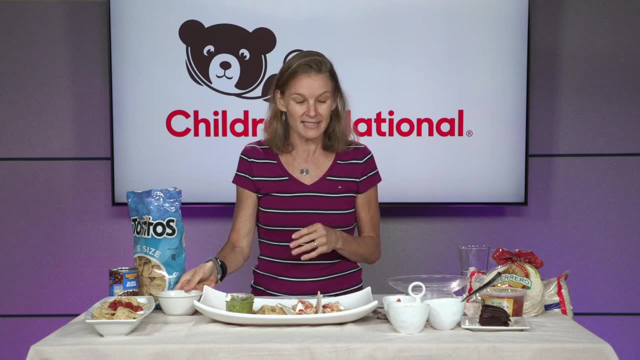 any of those low carb foods you want, and they don't require insulin. So what I could do in this situation is I could have some more of the chicken, I could top it with some of the tomatoes and the cheese and the sour cream, and even some guacamole and salsa. 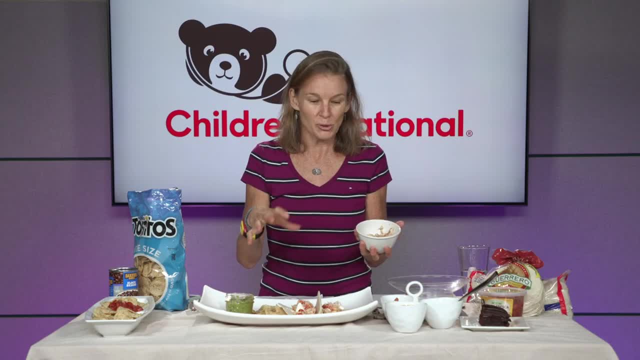 I could have almost a little bit of everything: A little burrito without the burrito, without the tortilla. So that's what I would do in this case. if I was still hungry. You can still have those protein foods and the veggies and some of those dairy foods. 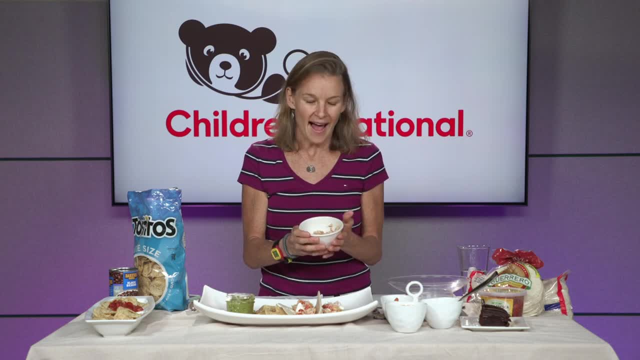 that don't have carbs. That way you don't leave hungry. If you wanted another piece of cake, you would have to take more insulin for that. So you've already had your nice size dessert. so you can add some more of those low carb foods. 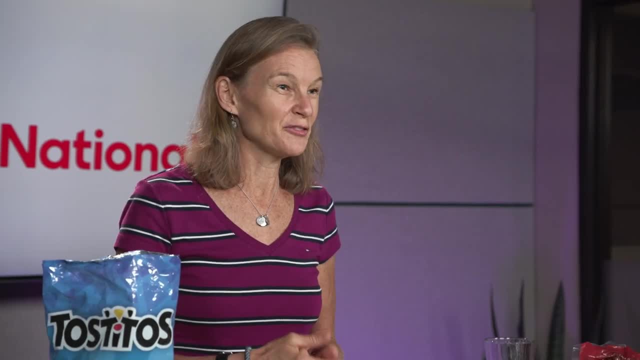 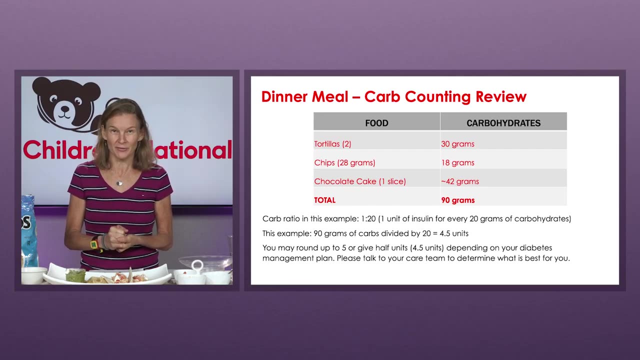 and be nicely filled up, All right. So what we're going to do this meal and how much insulin you need to take for it. We have our two tortillas. Those are 30 grams of carbohydrates. You had your tortilla chips for 18 grams of carbohydrate. 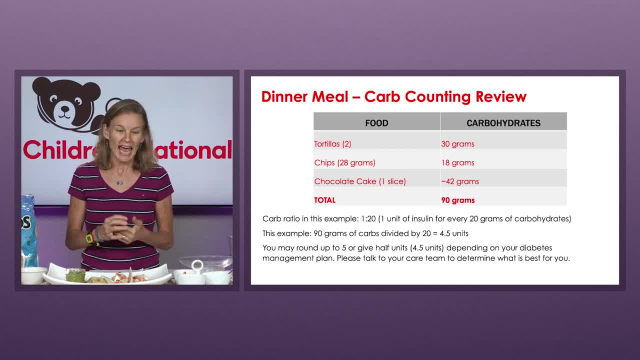 And then your piece of chocolate cake was 42 grams of carbohydrate. Adding that all up, that comes up to 90 grams of carbohydrate. What you do with that total is you'll divide it by the carb ratio that your provider has given to you. 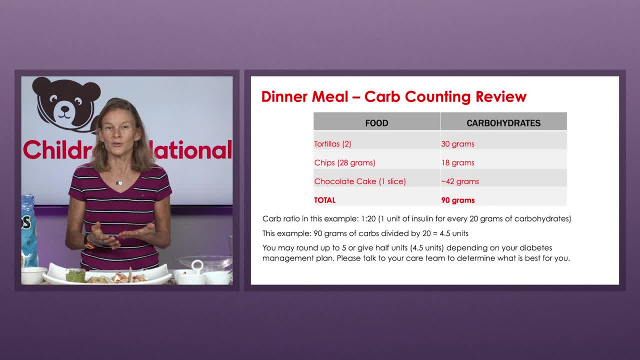 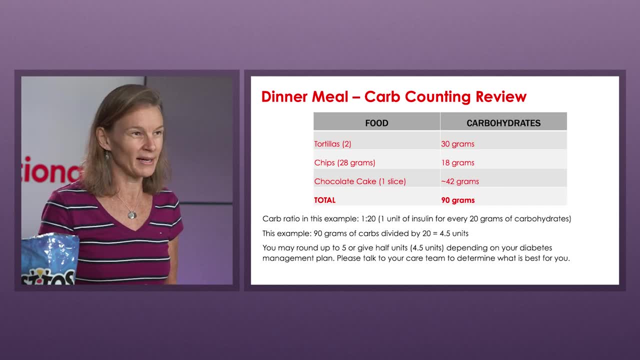 to calculate your insulin. So in this example we're going to use a carb ratio of a unit for every 20 grams of carbohydrate. So I'll take that 90, divide it by 20, and get 4.5. So I'm going to round that up to five units. 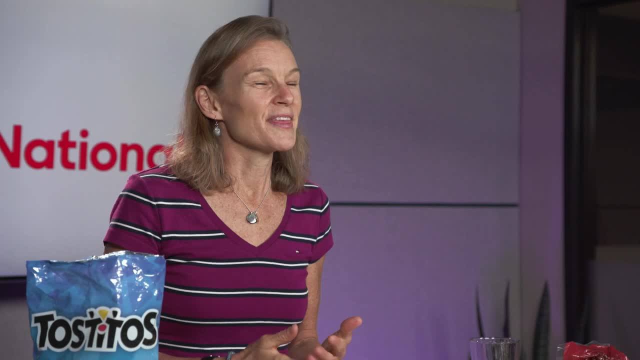 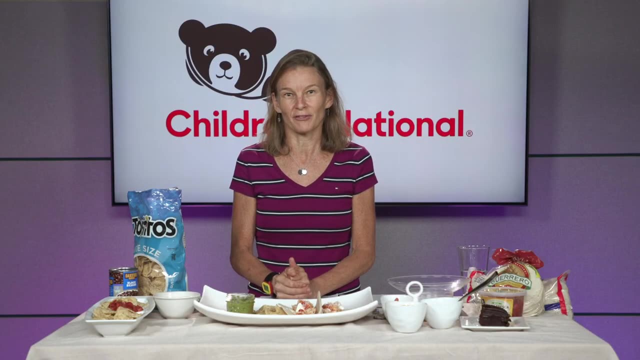 and I would inject five units of insulin for this meal. One thing you may find really handy as you're counting out these carbs in common foods that you eat in your household, is you can make a cheat sheet of carb counts and put it inside one of your cupboard doors. 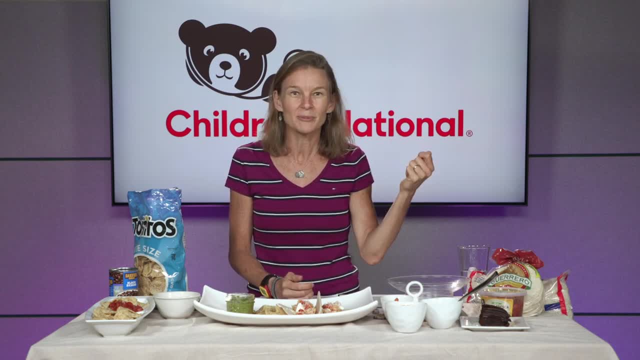 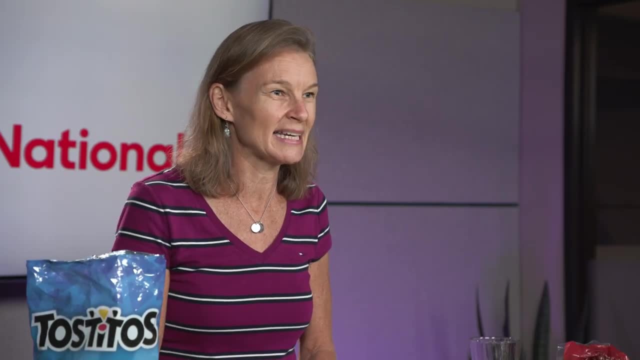 This is something I do in my house So I can look. My tortilla chips are always 18 grams of carbohydrates. Our favorite tortilla that I always buy 15 grams of carbohydrate per tortilla And you can have that list really accessible.